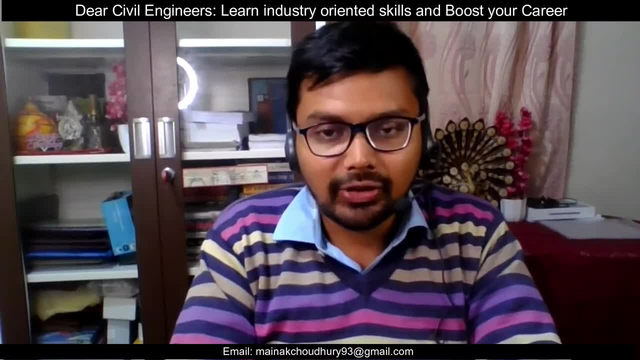 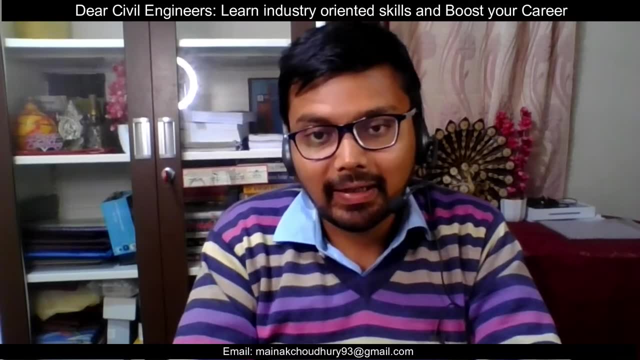 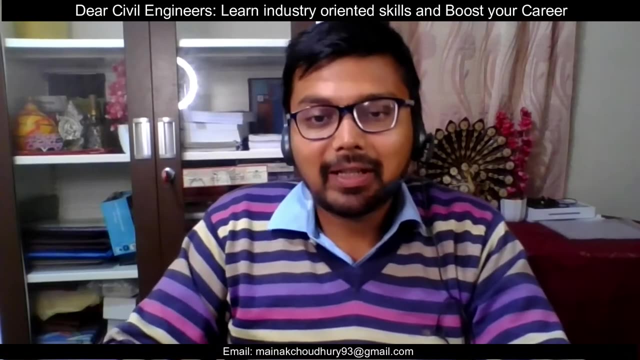 by part and as you progress in this video, uh just drop, like you can drop your progress, uh in the comments. and if you finally reach to the end and uh learn the software, you can drop a heart in the comments. and if you have any doubts, obviously you can ask in the comments and i will. 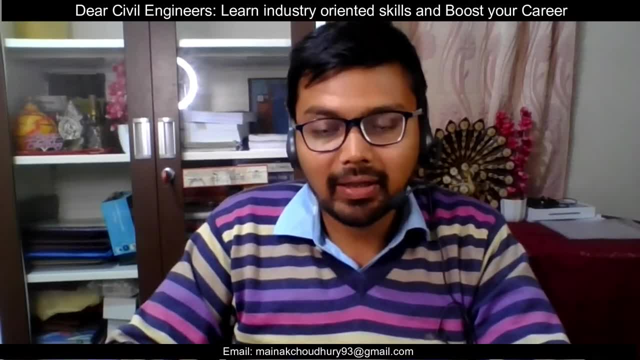 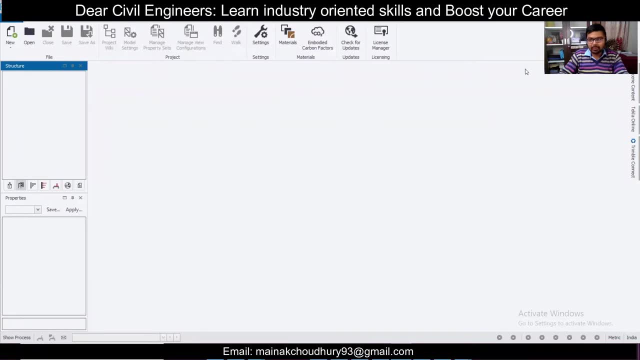 make a video on that particular doubt. okay, so let's start. so i had already made a video detailed uh series on eat apps, so i'll be using some reference there. i'll be uh giving the playlist link in the description as well. you can check out for the detailed explanation of the ios. 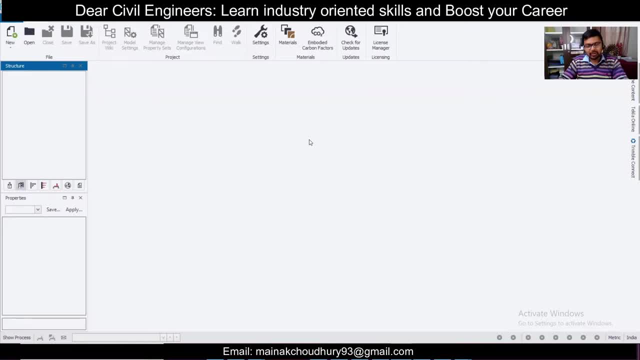 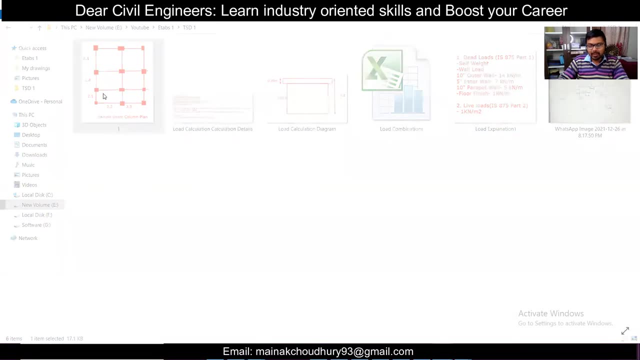 in this particular part, i'm not going to go very much deeply into the is codes, i'm just going to refer the all the things which i'm going to take. so first of all, uh, let me uh introduce to you the building. uh, you know your framing plan which we are going to make today. so this is the you know. 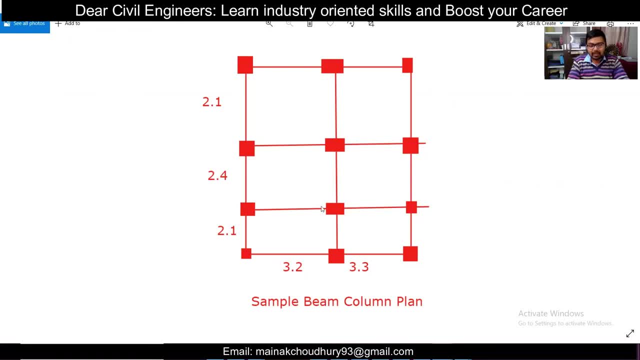 frame. uh, suppose you have an architectural plan. uh, you need to place the columns first and after they place the columns. you need to make this. you need to place the columns. you need to make this beam gunbildung. tecla does have a option of your importing the centerlines will get into that that. 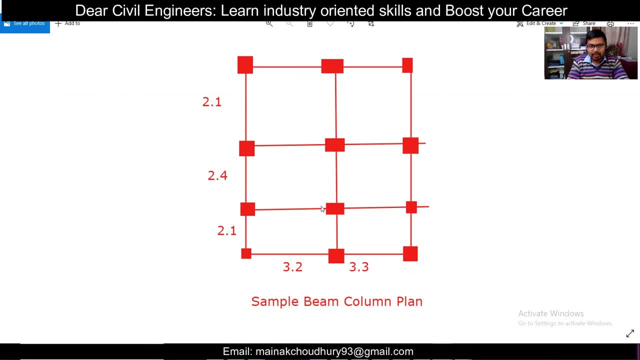 is a very easy feature, but, uh, overall, if you have this particular grid line, you can also do it directly in the software. so we'll be dealing with that particular procedure for that particular way rather today. okay, so we'll make this. okay, so this building will be, uh, you know, a g plus three. 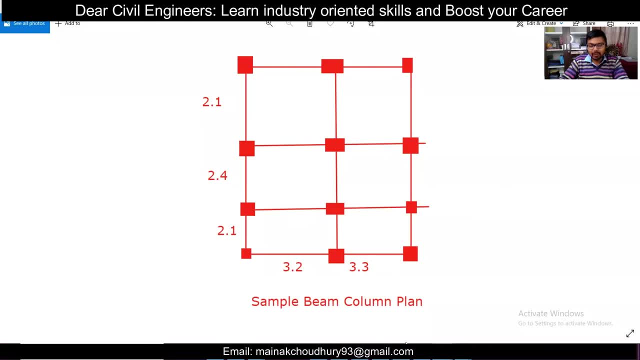 building, ground floor and three floats above this particular grid. so this is, uh, this, and there will also be the elimination of the texture and hair, so you can make a build in and, uh, you can have the different. you have victory from the series. so you know, the further it is going to have a panel, one interoco extreme. 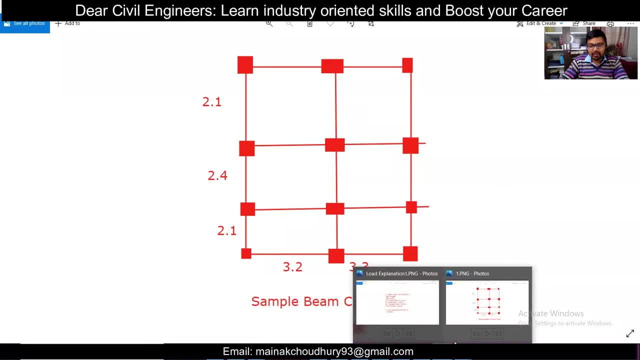 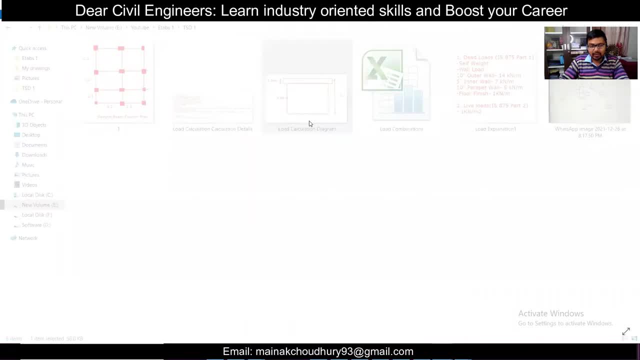 구tab so you can have in this series. so let's move on to improving the cielo. so let's take a look at the foam code. is the inclusion of the frame you could put, as we are going to take a look at each of the particular building and the height we can take as your 3.2 meters. so already you can see in the 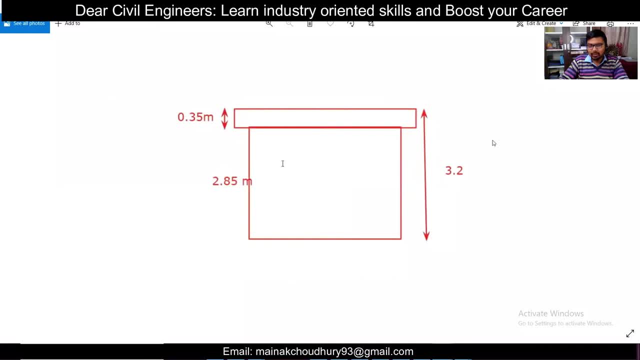 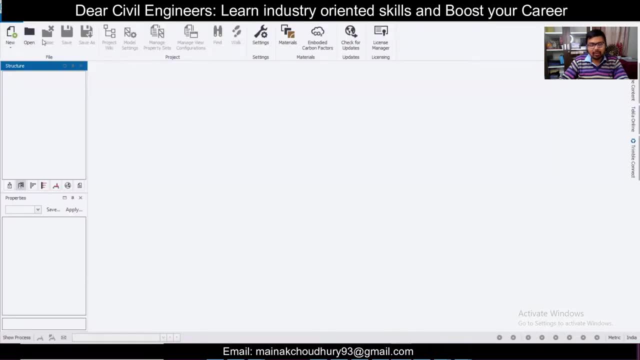 height of the building, height of the, you know floor to floor height you can take as 3.2 meters. okay, so we'll get into the details. so let's start. so this is the interface of the tecla texture designer. first of all, what you need to do is you need to click on new and, if you are used, watching. 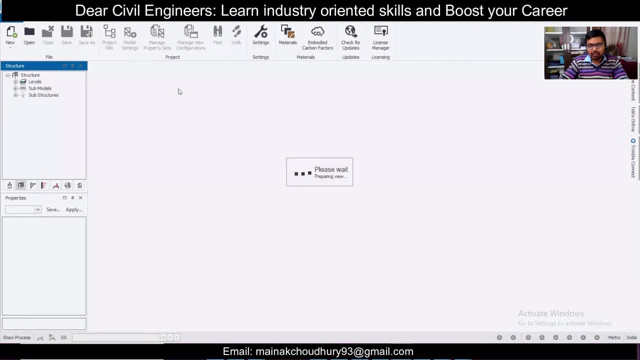 on YouTube. I'll suggest that you do the settings into the highest quality so that you know you can see all the icons in detail. okay, so once you click on new, the particular window opens up and you find one in structure 3D, which is obviously the 3D, and one is the base. so first thing we're going to do, 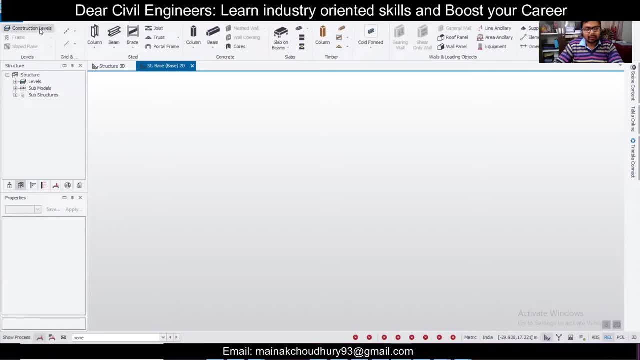 is we're going to make the levels, so we're going to go to model and then construction levels. so this is the base, as you can see, only level. so what I'm going to do, I'm going to click a- you know- insert below. so this will be a foundation level. now, the foundation level is usually taken. 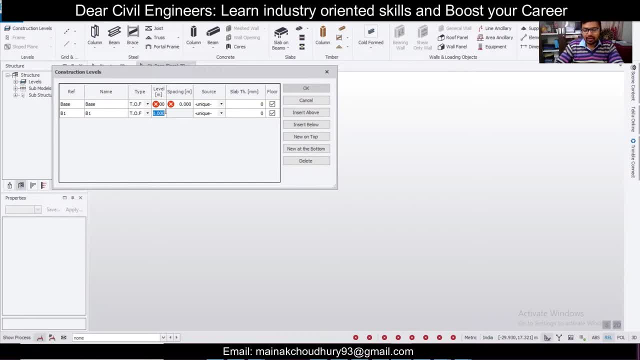 at a particular height. when, uh, and the geotechnical engineer or you know, you find the soil test report from any firm, then that particular soil test report gives you a particular SBC. at a particular depth, suppose at 1.5 meter, the SBC is: 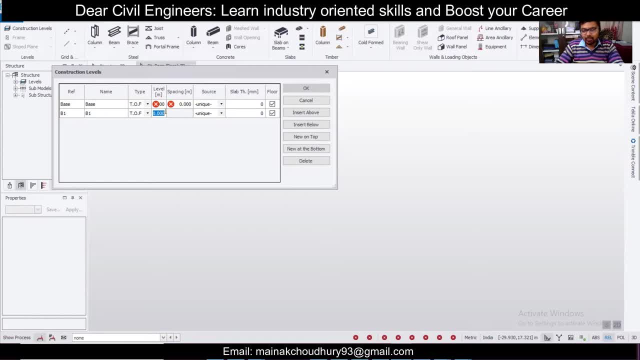 so, like this you do, so I'll do this as a minus 1.5 meters. that will be my foundation level and my plinth level I have fixed at zero. so zero is my plinth level or the base, and this is my foundation level and I'm going to let go a level above and this will be and the spacing which I'm 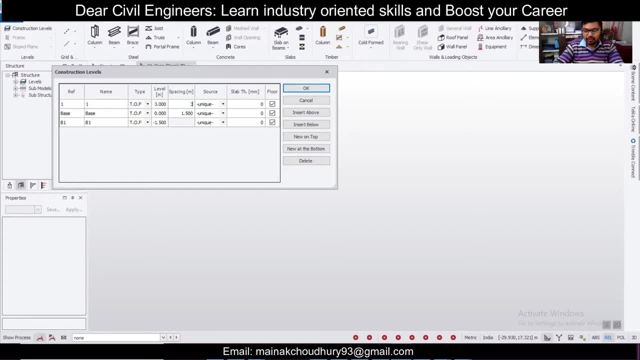 going to give here. uh is your uh 3.2 meters, so 3.2 meters for this, and this particular floor will be my ground floor slab, for my first slab. so this will be SSL, or structural slab level. tof means top of foundation or top of footing, and tos is used for the steel structure of steel. so I'm going to use SSL here. 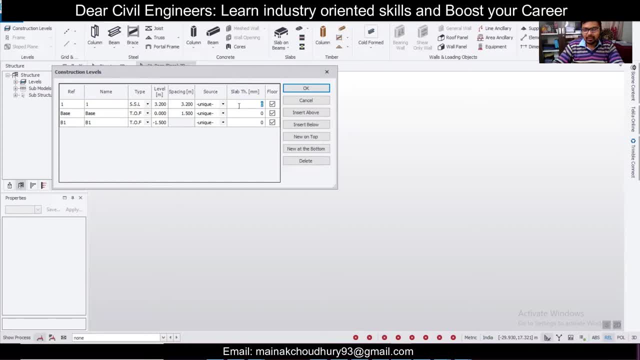 structural slab level- 3.2 meters- and slab thickness: uh, we know that we have to calculate the slab, so overall I'll provide a slab thickness of 150 mm. later we can change this, but now we are providing because by default in g plus 3 building it's between 125 to 175 mm. I'm giving going with 150. 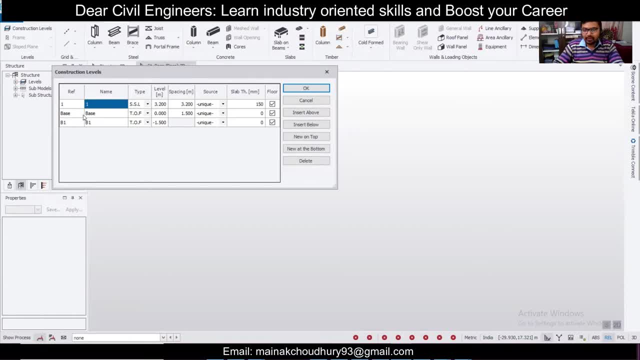 mm. okay, so a 150 mm slab thickness and my ground floor is ready. I want two more floors of this. I'll just click on insert above and insert above once again. so this is G, G plus one, G plus two. then you want G plus three, then another floor, so G plus three building: all the levels have been. 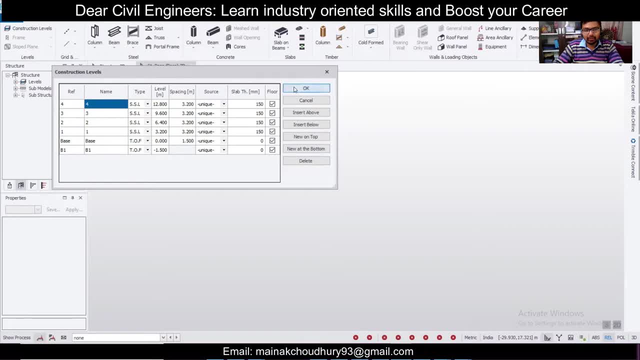 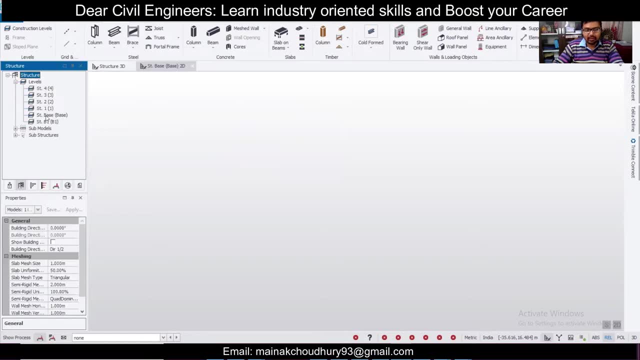 created. so after all the levels have been created, just click on OK. and now you will find here in the left side in the levels, there are all the levels. you can just go to any level by double clicking on it, suppose? uh, I already have to structure 3D and I know structure base open, so suppose I want. 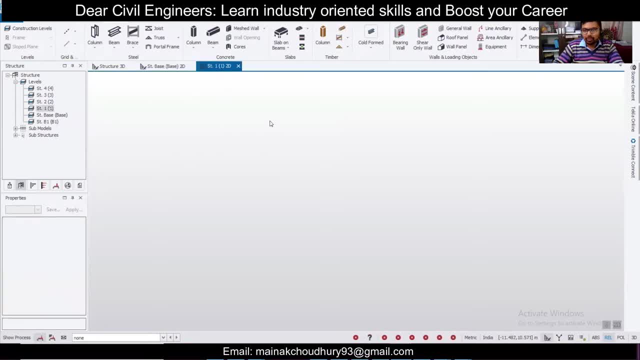 to go to one, I'm double clicking one and then I have one, two, three, four, five, six, seven, eight, seven, one. so like this you can go to any level. so let's go back to structure 3D. and now, uh, or, if best it is, you can go to the structure base, or we'll start at the plinth level and the plinth level will start. 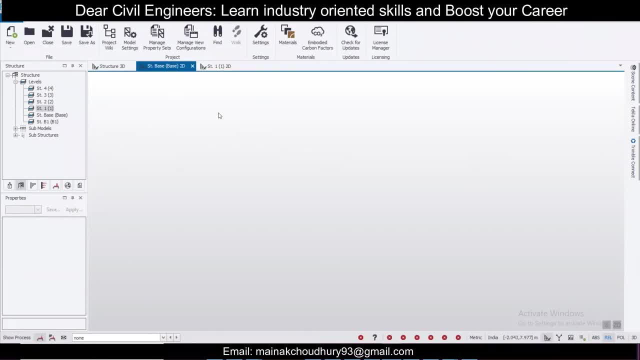 making our grids. so once we reached the print level, uh, using our diagram or the centerline plan, we'll just make the grid lines. okay, so we'll go to model and then we'll go to this option here and we'll use the rectangular wizard. so the first options don't matter, just click on. 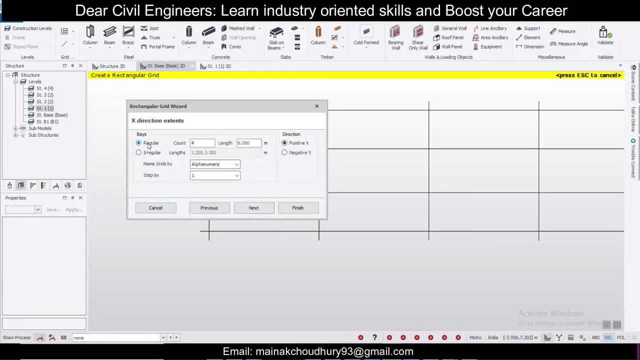 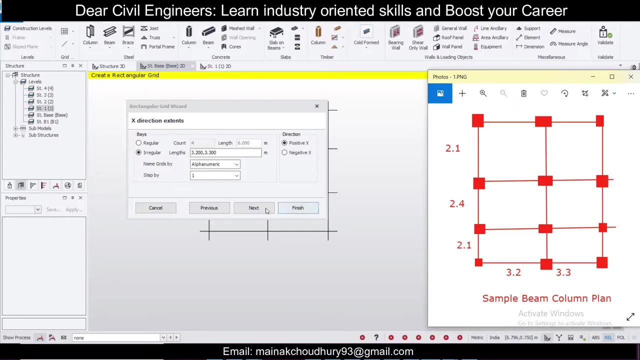 next here, and then you have this option of regular and irregular. so we'll choose irregular, and in the irregular we'll just insert here 3.2, comma 3.3 in the x direction. this is the extraction, and next then, in the particular y direction, we will give here 2.1. 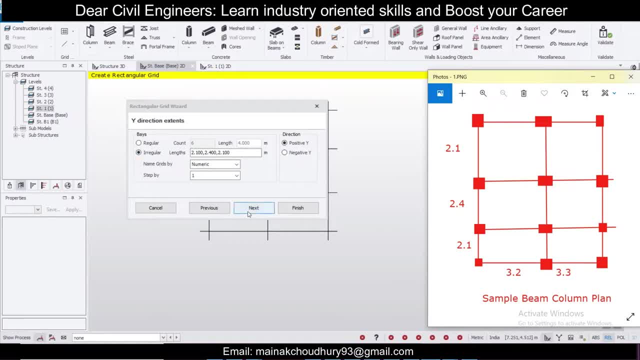 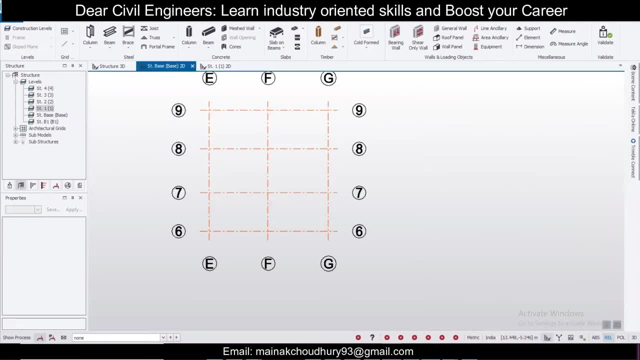 comma 2.4, comma 2.1, then just click on next and next and then finish, so we'll find the grids which has been created as per our diagram or the beam color plan. you can check here: click on measure, you can see this as 3.2. click on escape, again, just click on this 3.3, so you can see here 3.2. 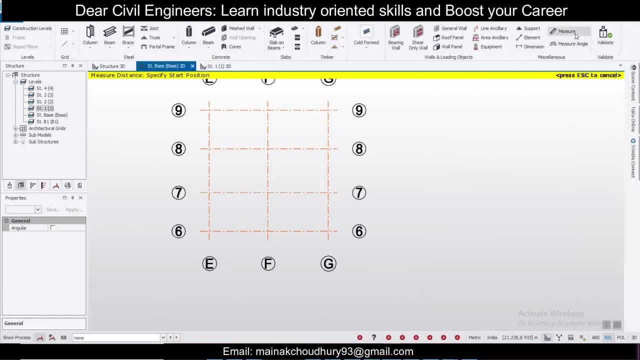 3.3, then 2.1, 2.4, 2.1. you just use measure again, select this and you can see here 2.1. let's click on escape this 2.4, escape, then 2.1. so our grid is okay and 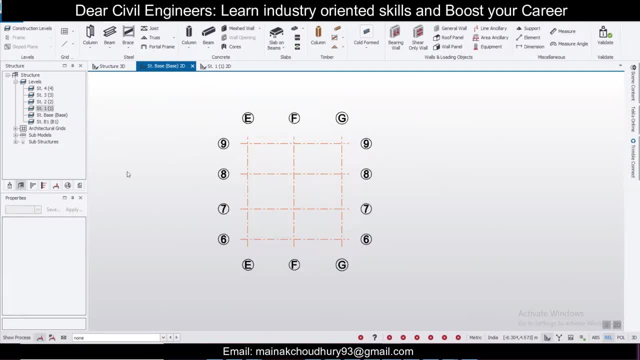 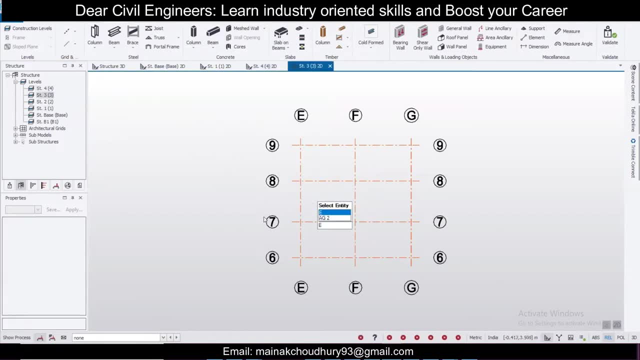 uh, this grid, if you see, has been copied to all the floors. I've clicked on escape and if you click on any floor, suppose the topmost floor I'm clicking on, so in all the floors the grid has been made here. so go back to the print level because we are doing operating from here. 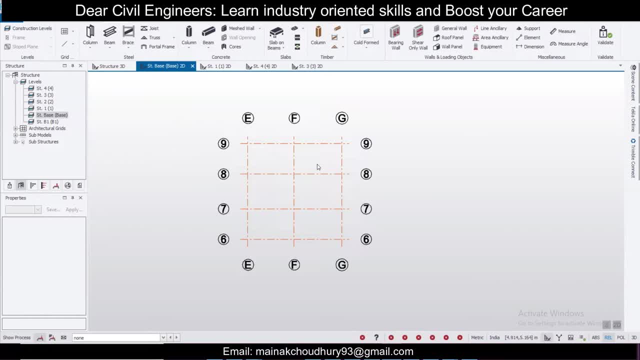 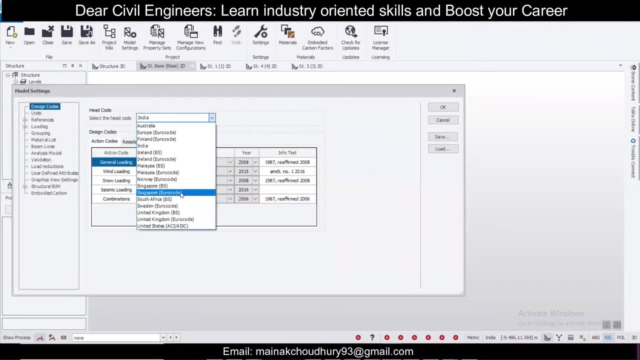 uh, in the print level, we want to insert the columns. so first of all, uh make sure you have selected the- you know- code of the country along which you want to design. so for that, uh go to home and go to model settings. make sure you have selected the country. here I am selecting India. 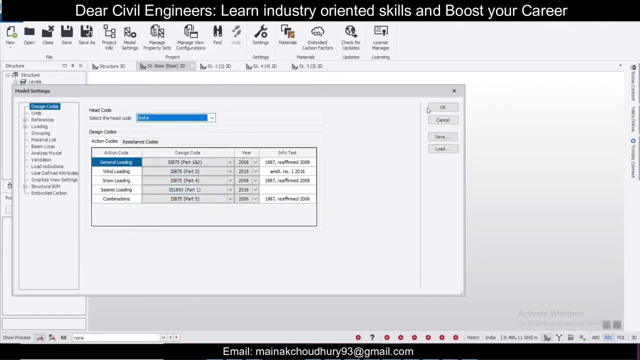 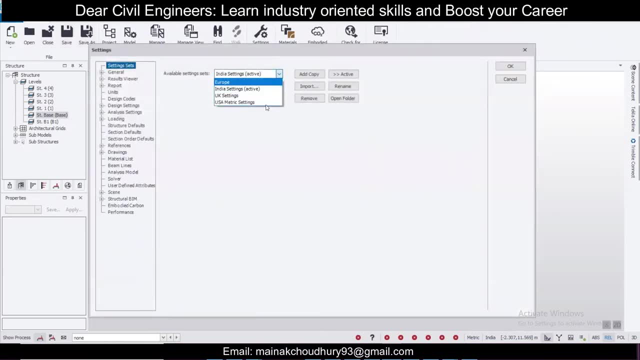 and you can see all the Indian codes for the building design have been selected here. just click on OK and save, if you are changing this, and then click on settings and here also uh, you can select the- if you want to go by UK settings or you can use the settings you. 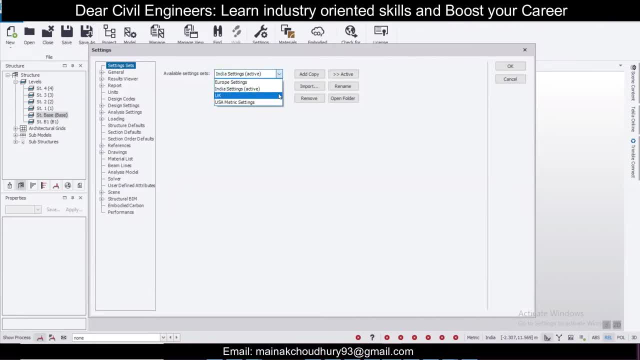 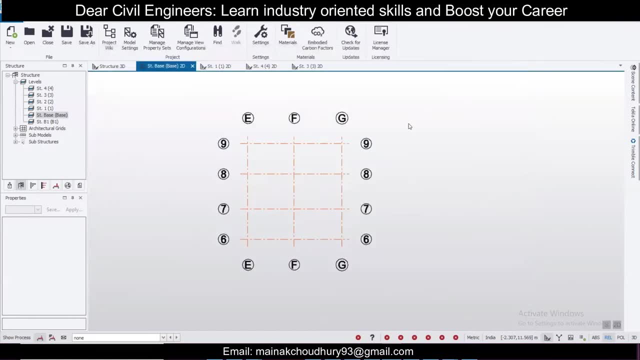 can do that. I have selected India settings, and if you want to add something which is not in this list, just click on import and you can find out the country. okay, so these are the basic things which you need to know. and then, uh, for adding columns here, first of all, go to columns. so I 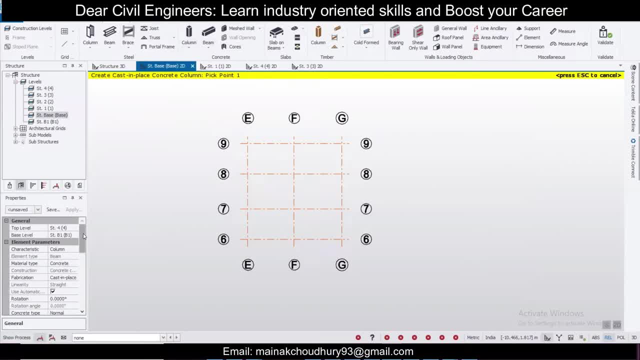 went to the models and then in the column. so, uh, what I'll do? I'll create a column first and I'll define the properties first. so let me go with 400 into 400 columns here. so here the size is already, you know, selected here: 400 into 400. if you want to edit this. 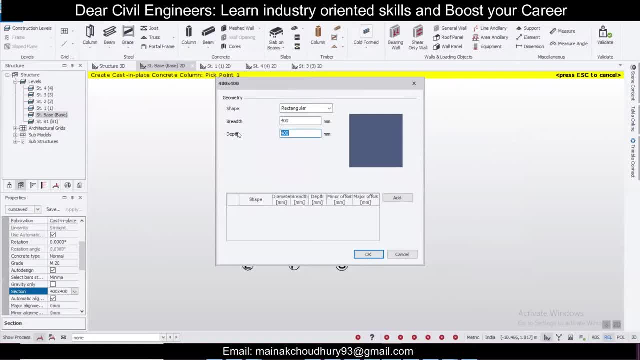 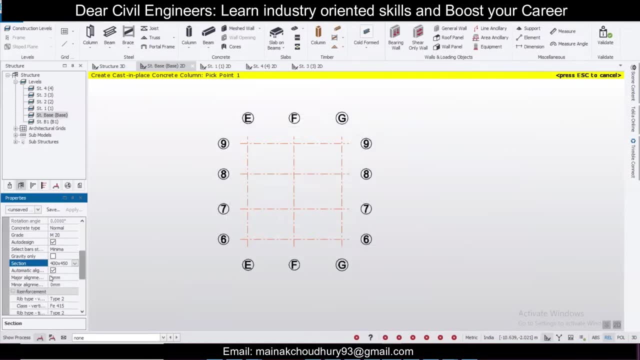 suppose you have to give any other size other than 400. let's, let me go with 400, 450.. so you go like this and click on OK, and uh, you, if you want to place the columns at the center, you just click on save and then you can make this as FB 500, the street rate and cover automatically. 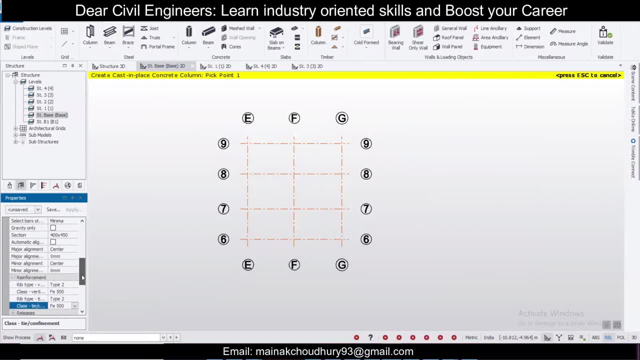 um, the takes as 40 mm, which is the default for the- you know, columns- grade of concrete. you can change M20, M25, so M20 is the minimum grade which is taken and most common. so you can use that and uh after that. after having everything, uh saved, just click on save here. so I'll do here. C 400. 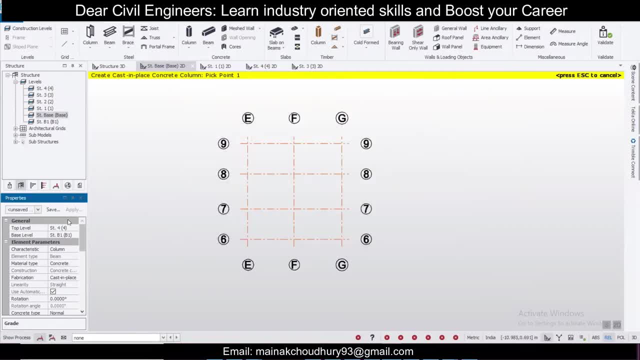 cross 450, just remember the name, and then click on OK and then select from here: see 400 to 450.. and then I can apply, you know, left click and apply it one by one in case I have different columns, or else I can just simply left click here like this and, as you can see, all the intersection. 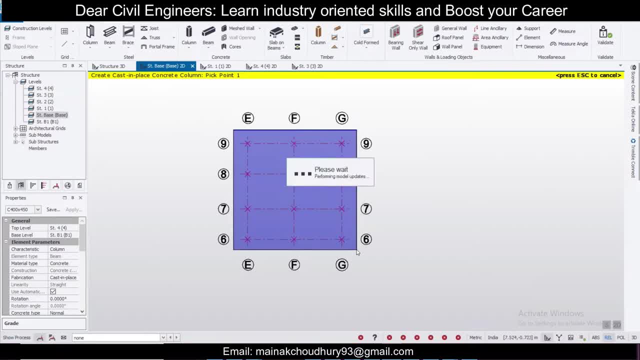 has been selected and the columns will be placed. so if I have like this, so it will be placed like this. so if I had separate columns, I'll just click control plus Z. if I had separate columns, would could have placed it like this: okay, one by one, and then i could have defined another column. 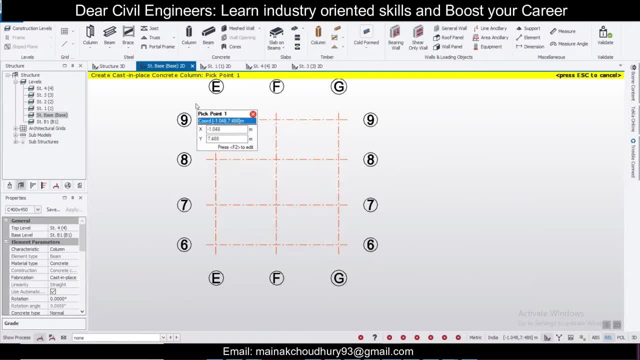 and then i could have placed- you know place- the remaining columns as well. so what i'm going to do is i'm going to just select all the columns and tecla has got a very, you know, nice user interface. you can see in the structure 3d and you can see this is mint. you can rotate this, just a right. 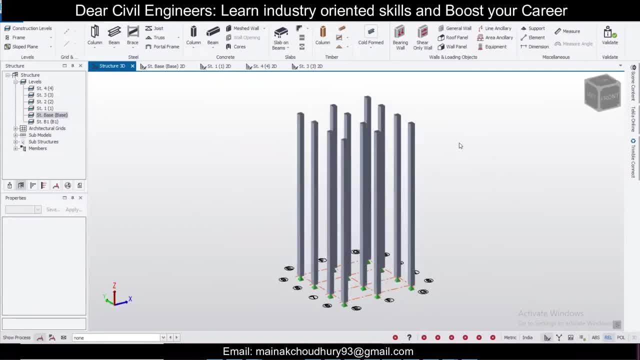 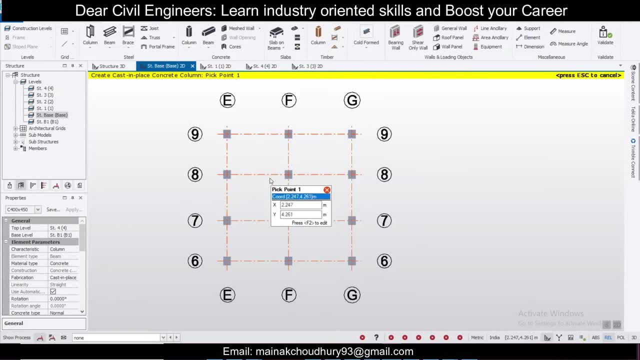 click on your mouse and you can see the columns which have been made. so it's very, you know, fine user interface. gui is very good here. so now, what you want to do, just click on escape. so next thing we're going to do is the beams. so i'm going to beams here and i'm going to define a beam here. 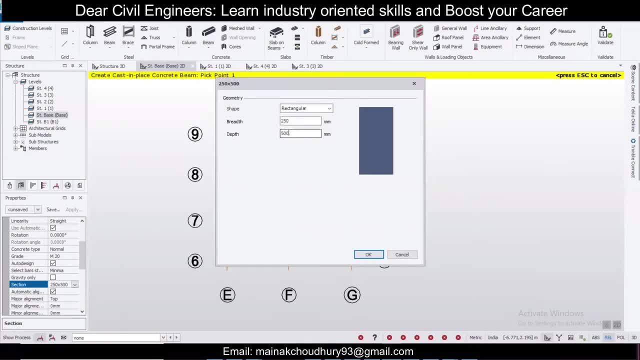 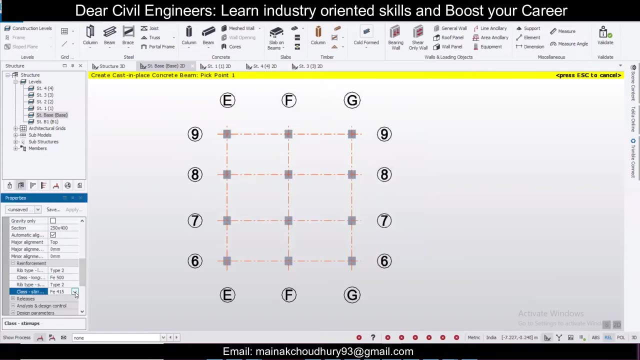 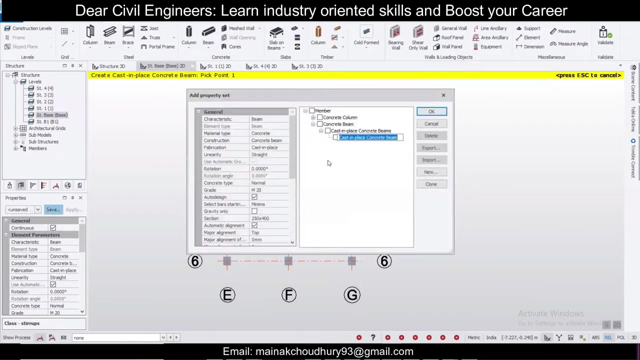 so beam size, i'm going to give here 250 into uh, 400. this will be my beam size and i will click on okay and after that just going to change this to f500 and also change this to f500, and after this particular change we will save this as b. 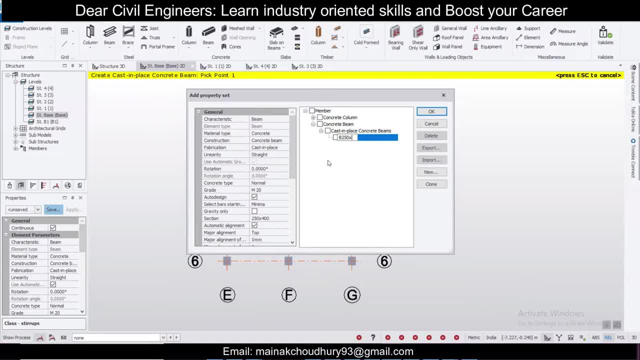 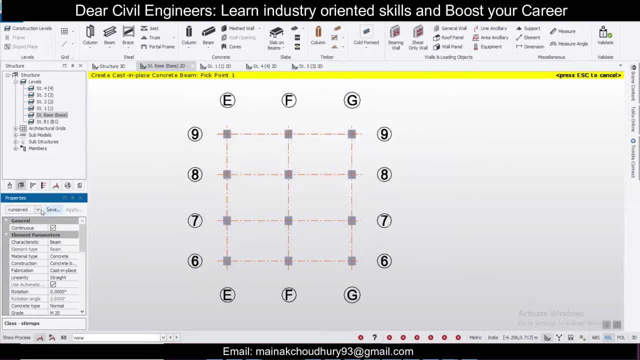 b 250, cross 400 and click on ok and after that you can select this b 215 to 350 and this is the print level. so the beams will be here. you can just left click here and then left click here, like double click here to join the beams, like. 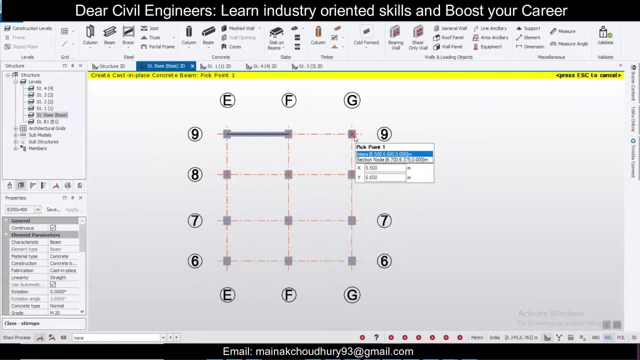 this. like this you can join all the beams. but if it is a column to column beam you don't need to join it. like this, i'll press control plus z and you can just simply drag it. like this it will be joined and in this case, since all our column 2 column beams, i'll press ctrl plus z again. 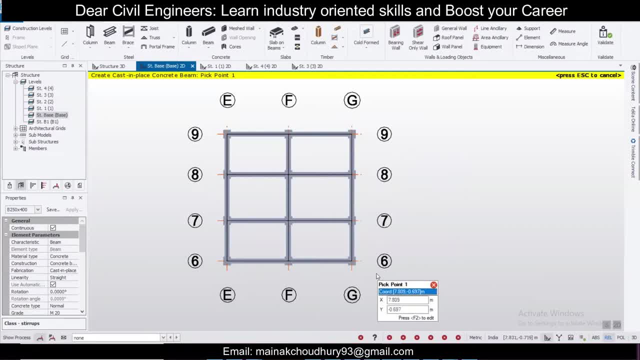 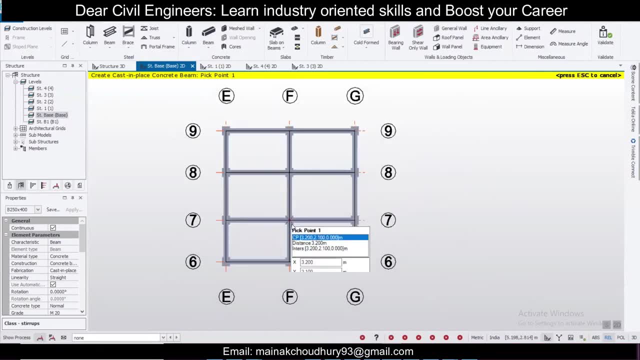 we simply drag it like this and all the beams will be joined. so in all the positions where your beams you can join the beams you know. where you have little bit more complicated beam column diagrams you need to play, you join them one by one. we'll go into that where we uh make our full project videos. 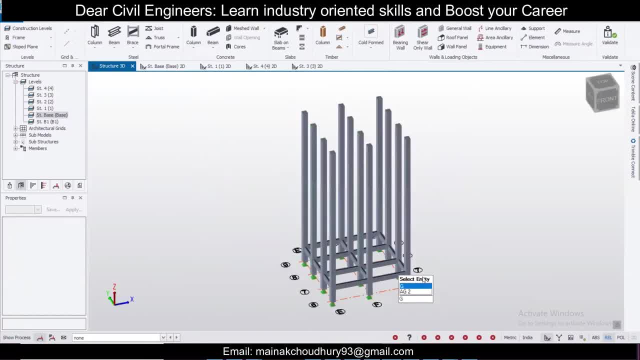 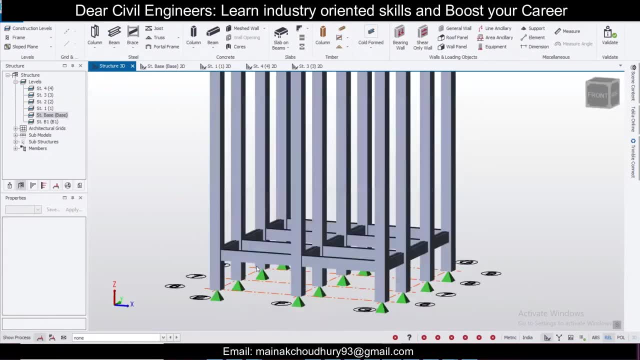 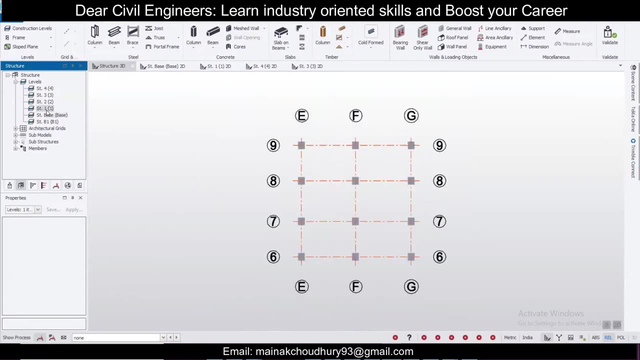 so now you know how to make the beams check out in the structure 3d. this is the beam which has been made, so we'll go to the next level. since this is the plane level, it will don't have- uh, doesn't have- any slab, so the next level we'll just go to structure one. so this is my next level and select. 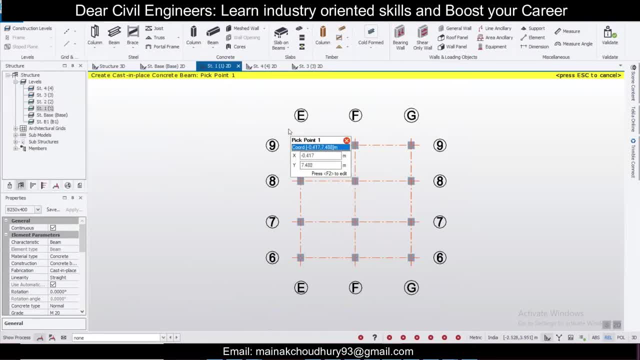 the beam and i'm going to take the beam section and i'm going to same way. i'm going to apply the beams. next, what i'm going to do, i'm going to click on slab automatically. you know, 150 slab will be taken just left. click on them and the slabs will be taken. here, two-way slabs are taken as default. 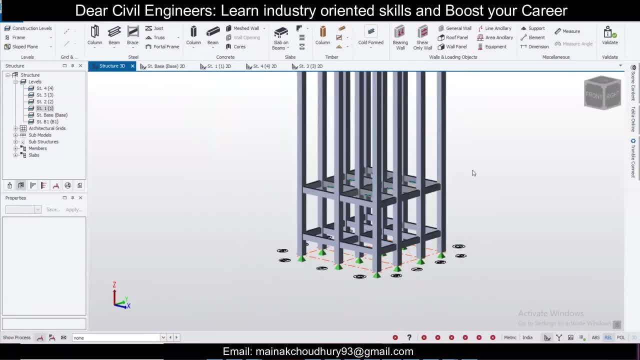 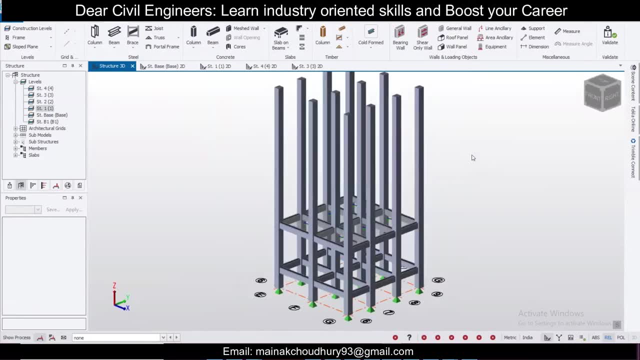 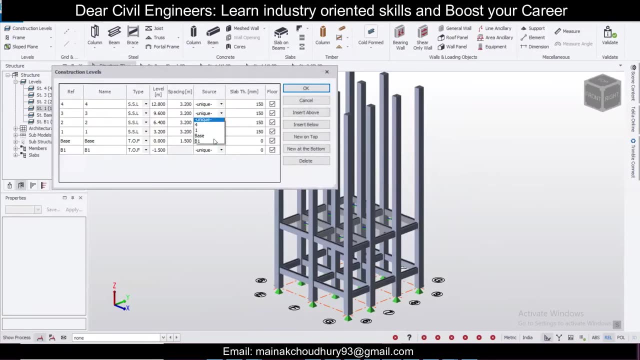 as you can see, slabs have been provided. so now this particular thing, i can copy to all the remaining floors, since all the remaining floors will also have the slabs, so i can go to construction levels and make this source as one, this also one, and this also one. one is the level for the ground floor step level, which i have just 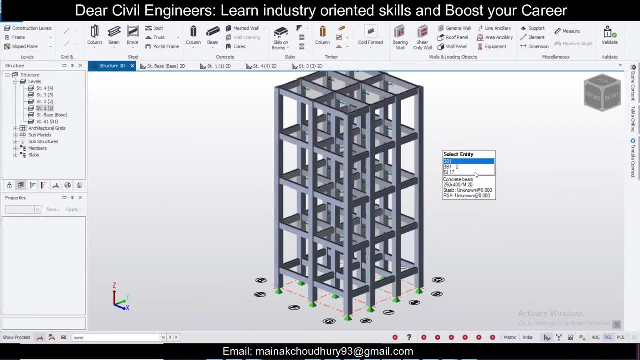 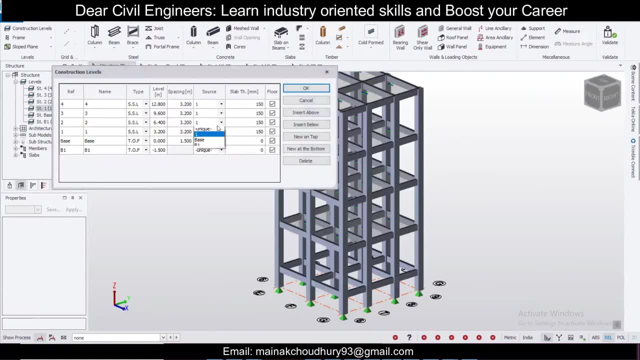 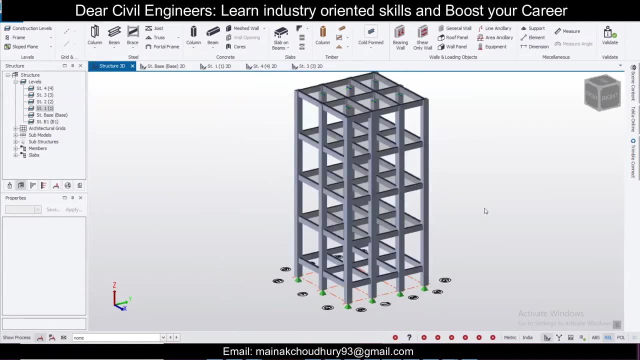 created. so if i click on ok, this particular tool will be copied to all the flows in a single go. then we can go to construction levels again and quickly make this as unique, because all the changes which we'll do in terms of the loading, we don't want this to be copied to the other floors. so once it is unique, 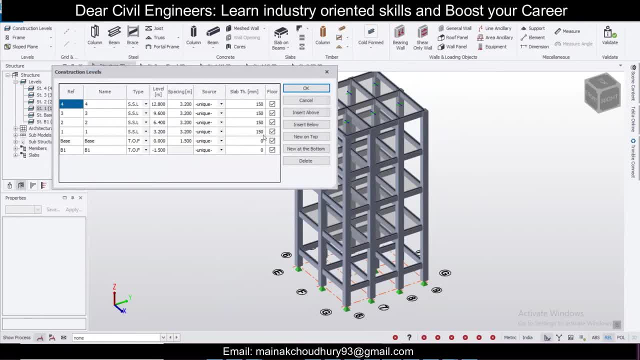 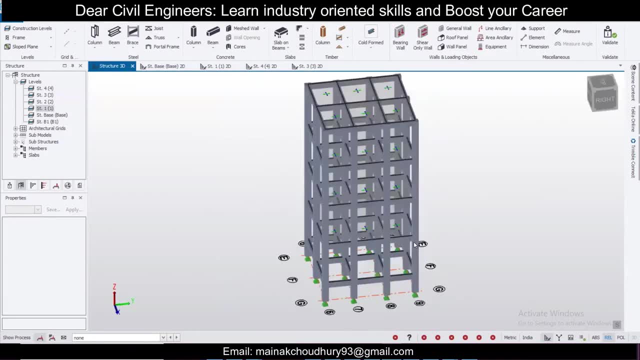 go back to construction levels and check that all are unique. this check is very important, but sometimes you might forget to make them back as unique. next thing is about the loading part. so the loading part. i'm not going to take much time. as i've already explained in the etabs videos about 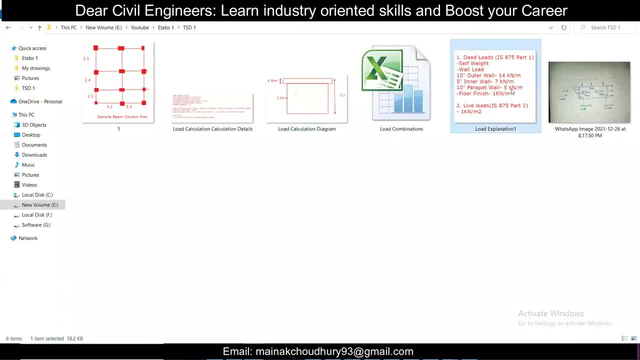 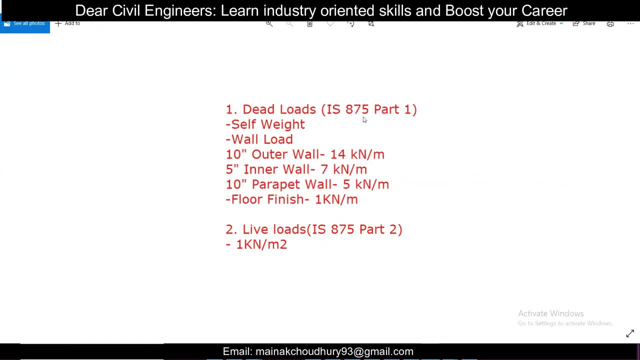 is codes and how to determine the loads. just, you can take a screenshot of this, of what are the loads we're going to take in terms of lead loads and live loads, dead loads. the code for it is is 875, part one. you all know that. if you don't know, just remember this and also watch the. you know. 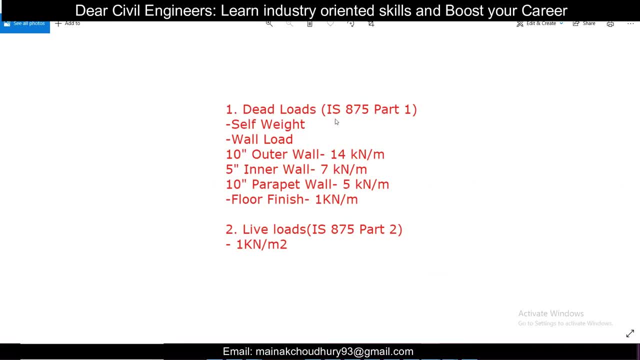 video in the etfs part so that you can know what are the basic things you need to remember and basic things you need to know about this code. so self-weight, the software automatically takes one load. we're going to put in the particular software for 10 inch wall. we're going to give 14 kilonewton per meter. five inch inner wall: seven kilonewton. 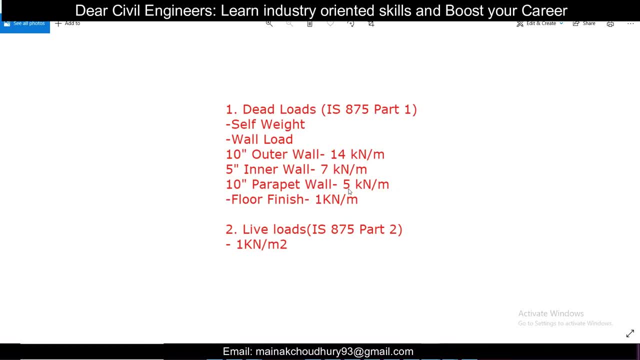 per meter. for the parapet walls we'll go for five kilonewton per meter and floor finish load overall we're going to apply one kilonewton per meter for the floor finish live loads. we're going to take here two kilonewton per meters but there's a i know mistake, so it will be two kilonewton per meter. 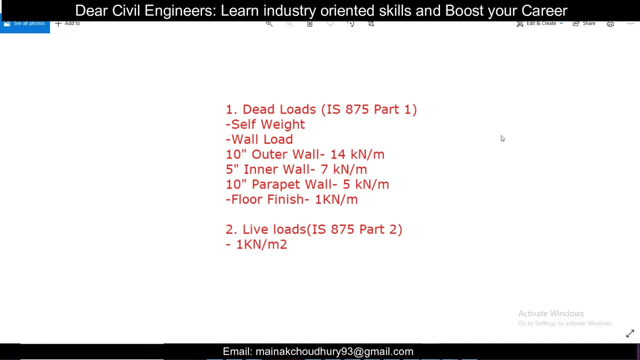 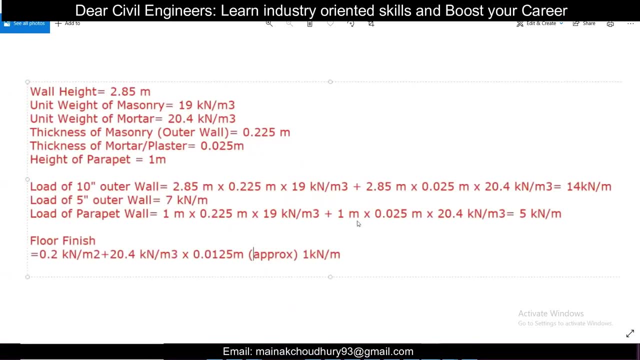 squares per is 875. part two for the residential buildings. the detailed calculations are also there. uh, you can take a screenshot of this. uh, detailed calculations. or if you want to know the explanation, go ahead and in the etf playlist you can check the part on the dead end live loads. okay, so you can do that, so we'll. 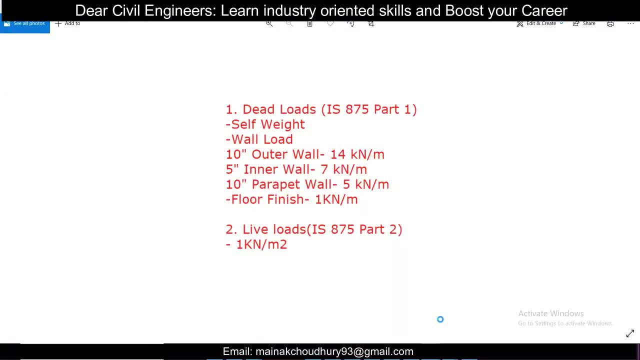 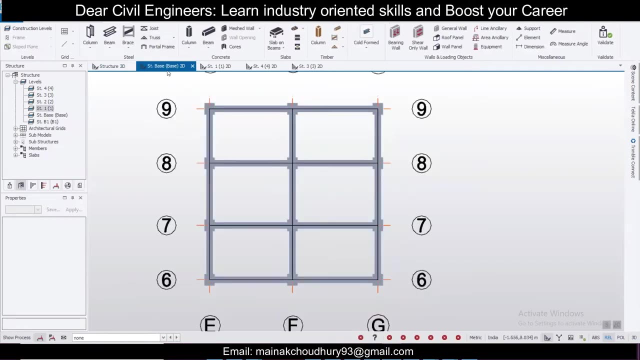 just apply all the loads as per. you know this, okay. so first of all, let's apply the wall loads 10 inch wall load 14 and inner uh seven and for the parapet five. so let's do it now. first of all, we're going to go to the base and we'll select here dead, and after selecting dead, uh, we'll go. 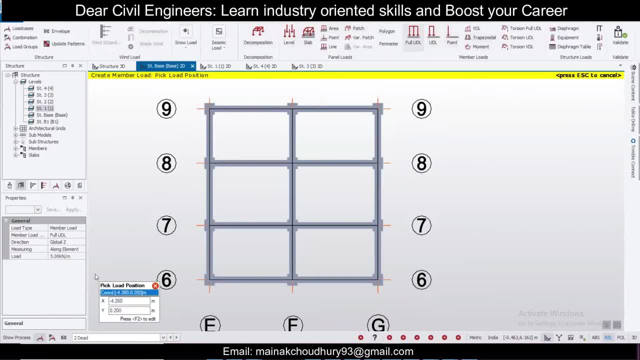 here with you have this load option: full udl outer. let's go with 14. okay, just left click, left click, left click. so we're going to left click on the all the outer beams where the outer walls will be there. you can check here in the bottom right. uh, there is an option, click here. so 2d to 3d. 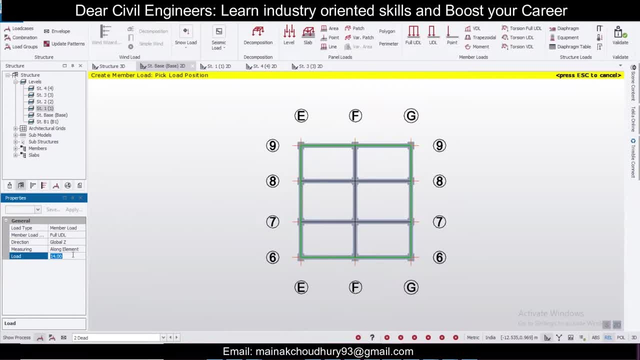 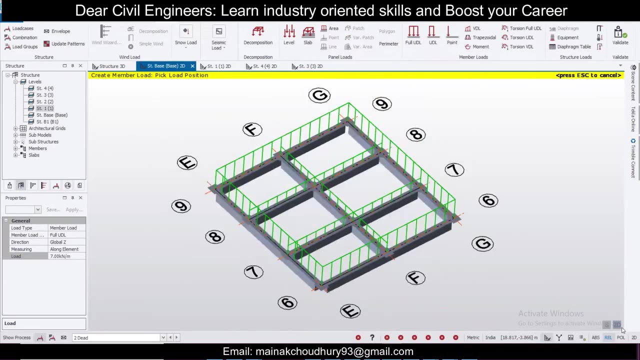 we'll check. the 14 kilonewton load has been applied. so now we'll change this to 7 and then apply it on the inner walls or the beams on which the inner walls will be there. check back 3d and notice the level of the difference. so similarly, we'll go to the one here. 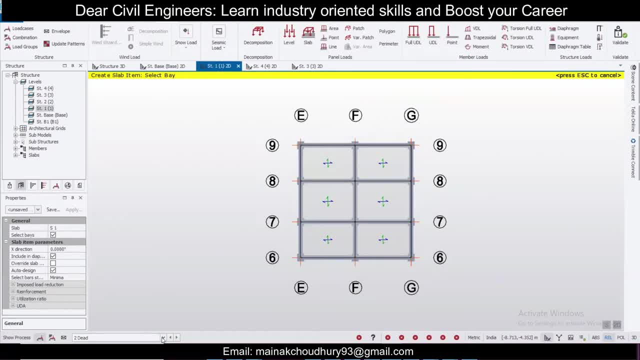 and here also we'll apply the select the dead load, full udl, and here also there will be 14 in the outer for the 10 inch walls and plus 5 inch walls go with 7.. so load calculation: if you know how to calculate it as per your varying wall thickness, you can calculate the loads. so in the dead loads, 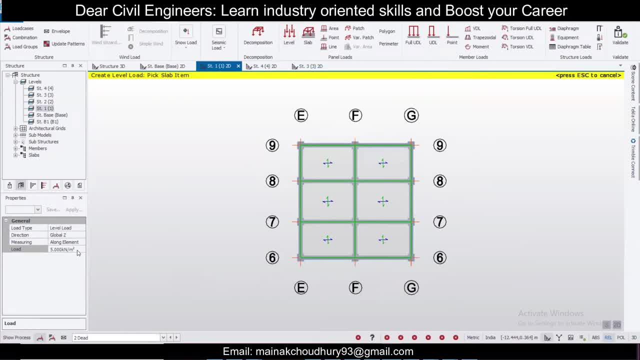 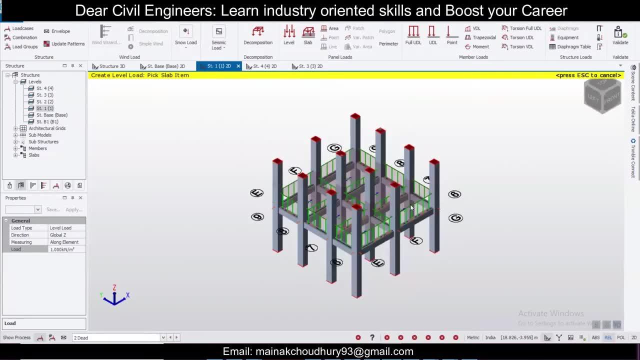 also i'll go with level load here and for the floor finish i'm going to get like one kilonewton per meter step. so i've selected this so as you can see floor finish off, then you can escape floor. one kilonewton per meter square has been applied and the wall load has been applied in this. 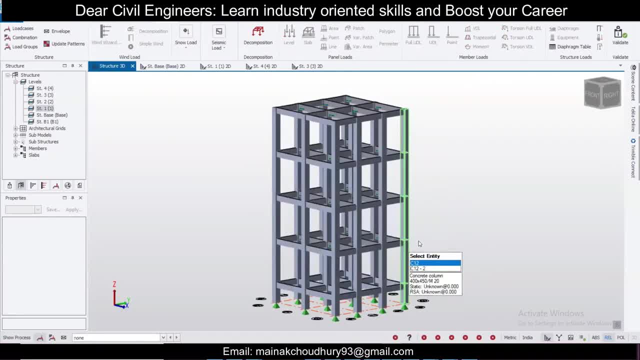 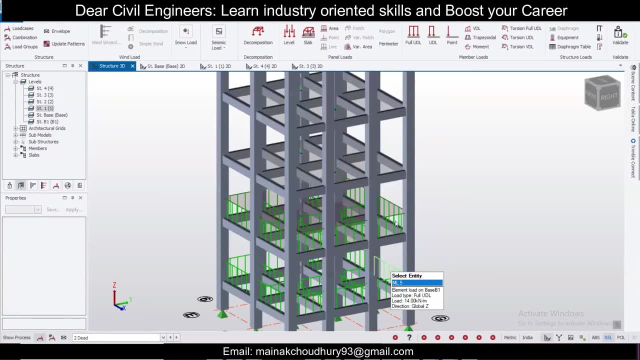 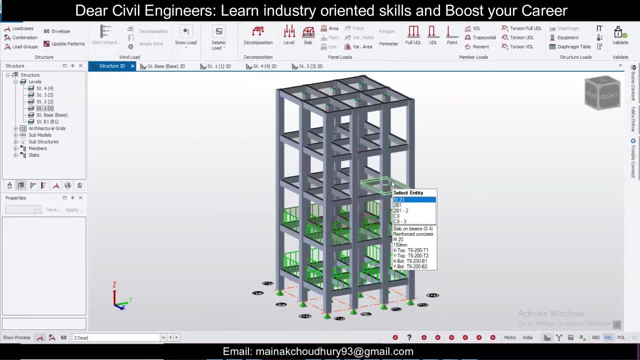 particular level. so in the structure 3d i'll go here and i'll just select here, you know, dead load. so, as you can see, this is the particular dead load which is in this particular flow. if i copy in this two next two floors, i can do this, i'll go to model, i'll go to construction levels and for this two i'll make this one. 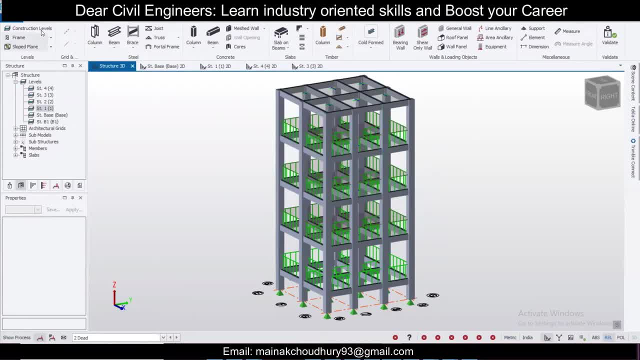 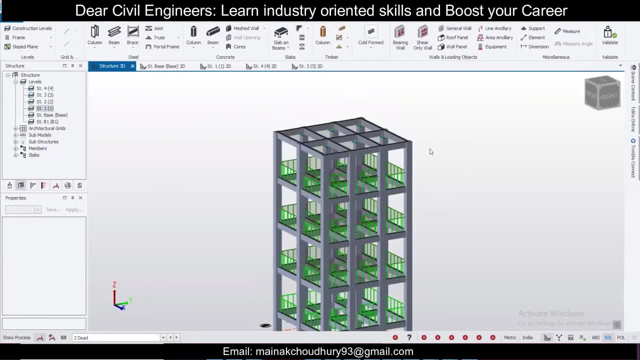 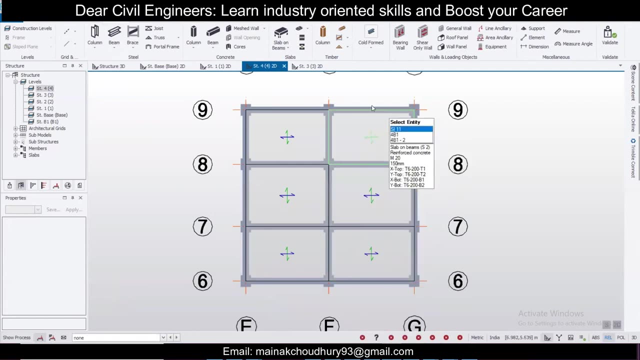 also this one. click on ok. so these loads have been copied. go to construction levels and make them back as unique. click on ok. so in the top floor i'll go here just level. click on structure 4, top floor. i've gone and for the parapet wall, only along the parameter i'll apply a load of five. 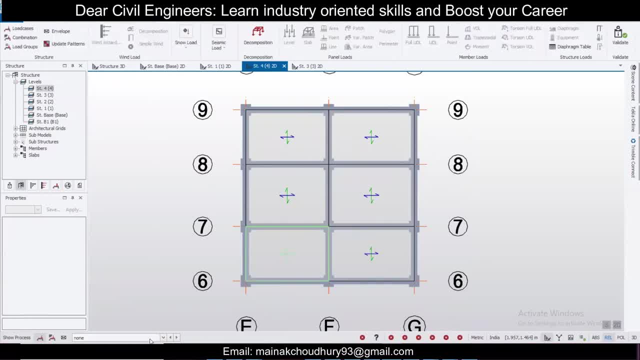 kilonewton per meter. we're going to load and selecting here dead load, full udl of five left and apply it for the parapet wall and also floor finish load. uh, you know it don't need to apply on it here because this will be a. 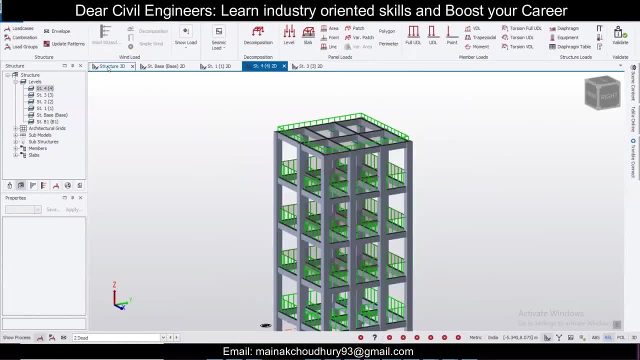 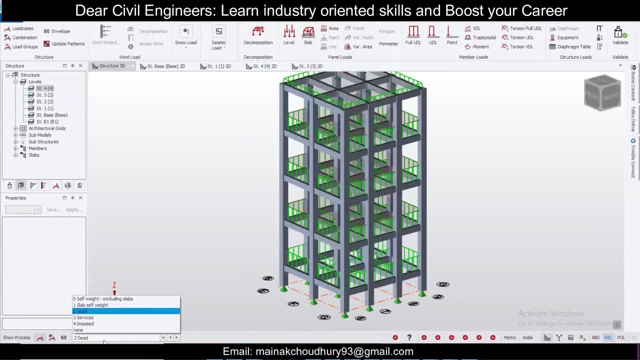 roof. so no need to apply the pro finish load. now you go to the structure 3d and you can check here the loads which you have applied. so we'll switch back to the imposed load and we'll apply the live load here. so you take a level load here of two kilonewton. 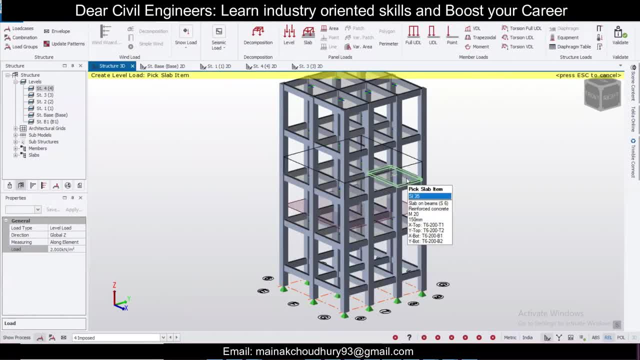 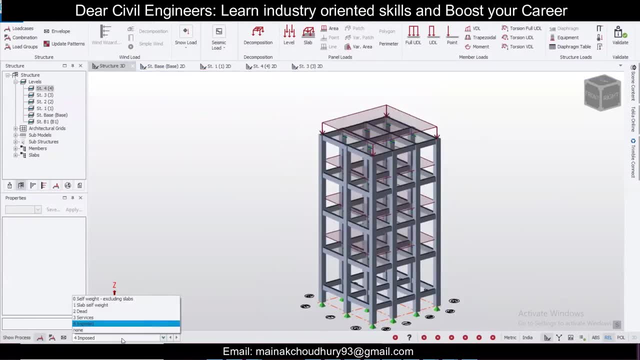 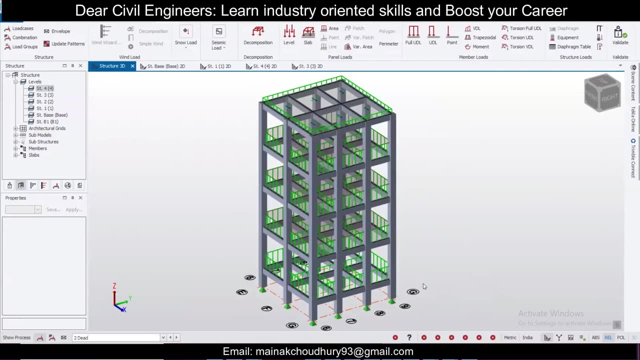 per meter square. so we'll apply it on all the floors, the live load. so once the live load has been applied and also the dead load has been applied, so you can go after this and you can take a break, and you can come after the break you can take a cup of coffee. 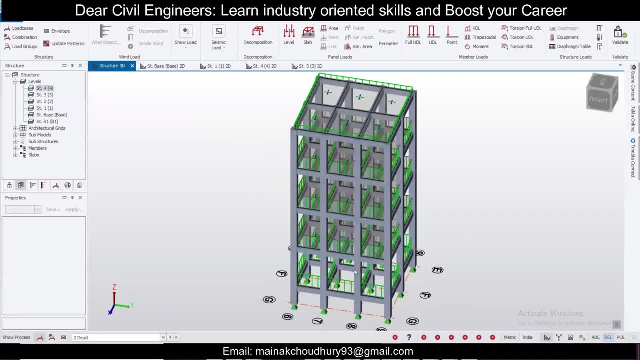 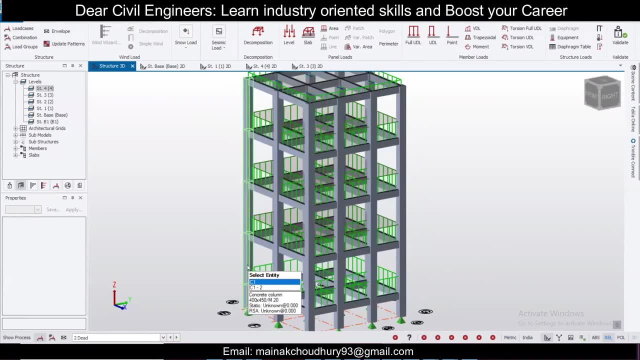 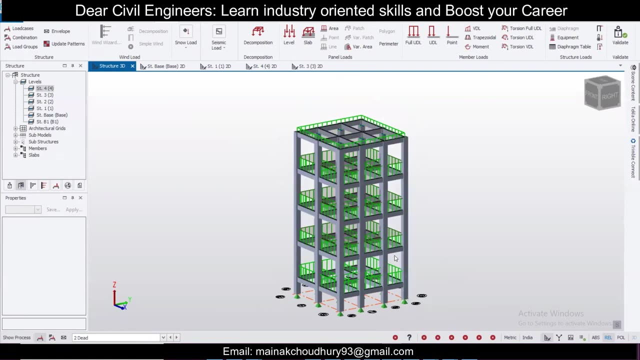 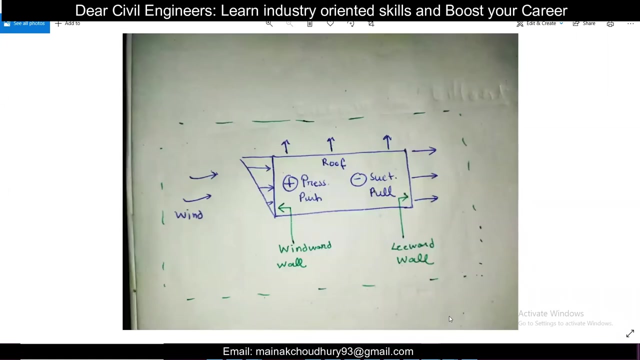 and come after the deck. so, welcome after the break. and now, uh, what we'll do? we will move further into the other looks, which is the wind load and the seismic load. so explanation detail i have given for the wind load and as well as the systemic load, which is 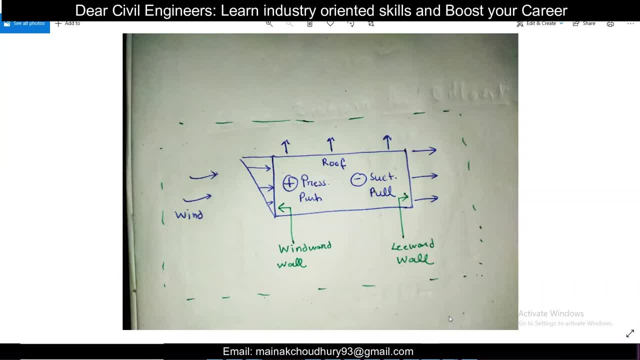 wind load code is 875, part 3, and basically, if you see, this is a building and the wind is acting here. so wind is a lateral load. so the direction in which the wind is acting it is, uh, you know, windward wall and the opposite direction is the leeward one. so there are wind coefficients which you need to apply here. 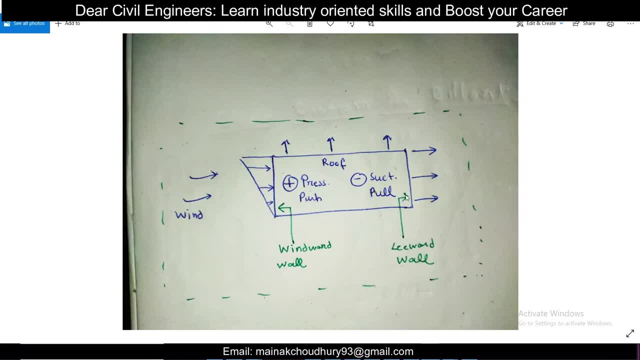 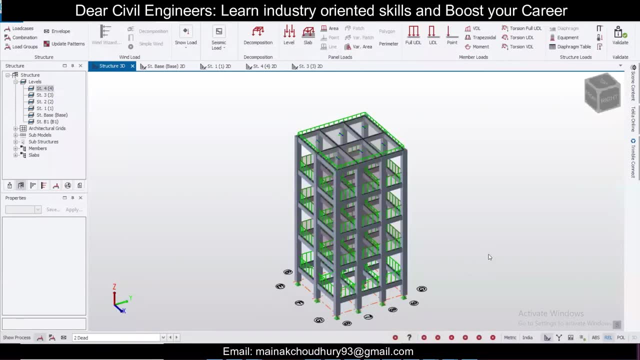 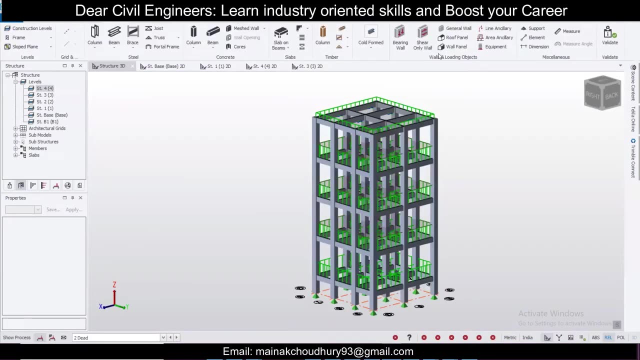 and this is basically on the windward side. this is 0.8 and the leeward side is 0.5. so you're going to remember that and all the other details i've explained in the etabs videos or the is code part can just go through that. so in 3d view, what we'll do. 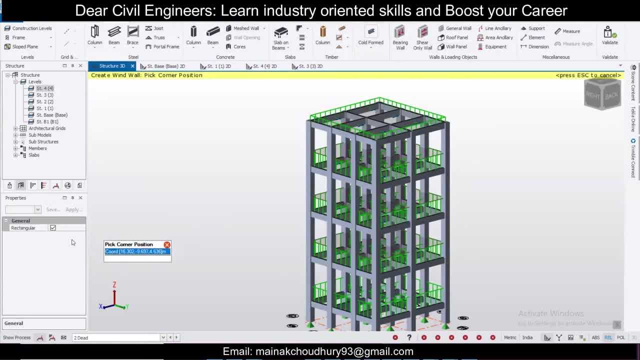 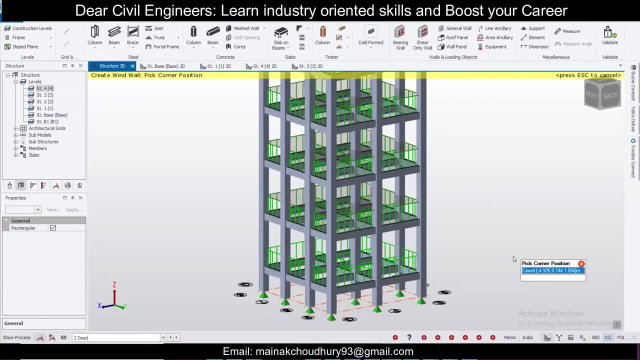 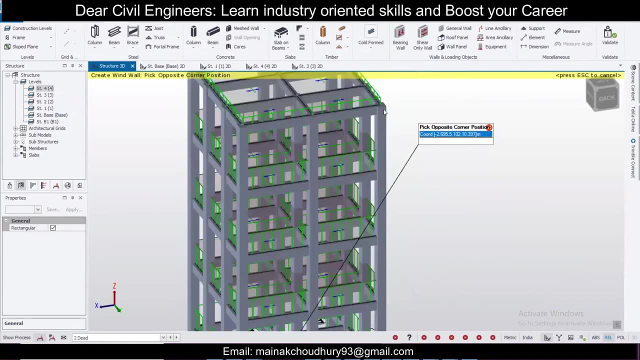 is, we'll go to our model and then we'll make our wall panels so rectangular panels have been selected. uh, right click and obtain a suitable location for selecting this corner selected and then this corner. as you can see this corner if you select this, uh, selection is not. 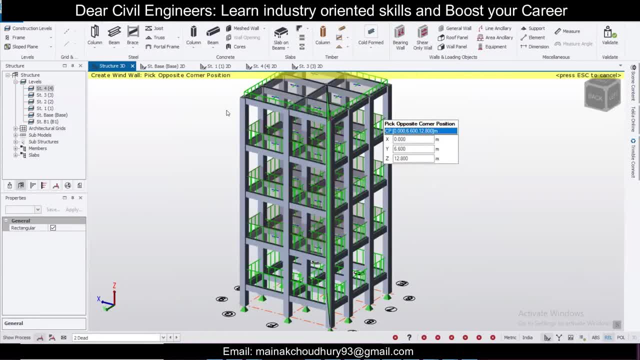 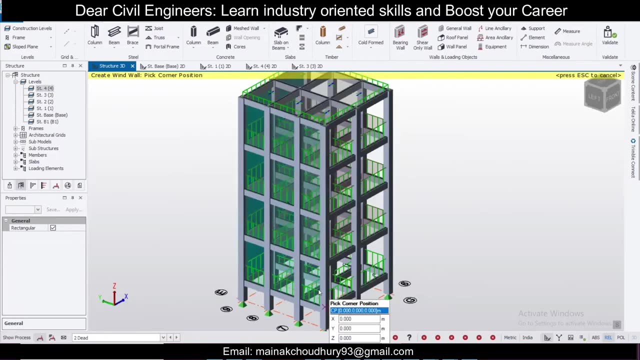 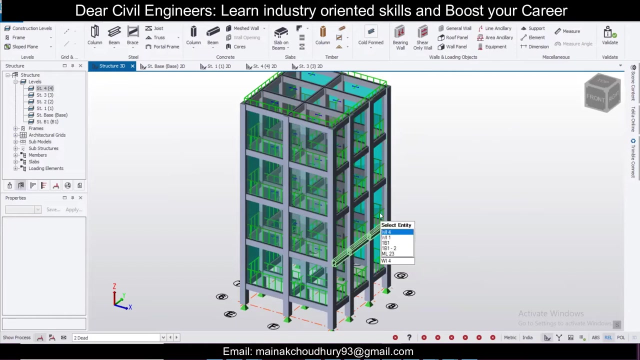 happening properly. you can see that. so rotate it properly and after that this clip on escape and then select a proper location and then select it like this, really do like this: rotate and then select and then select. like this, select and then select. like this we're gonna skip. 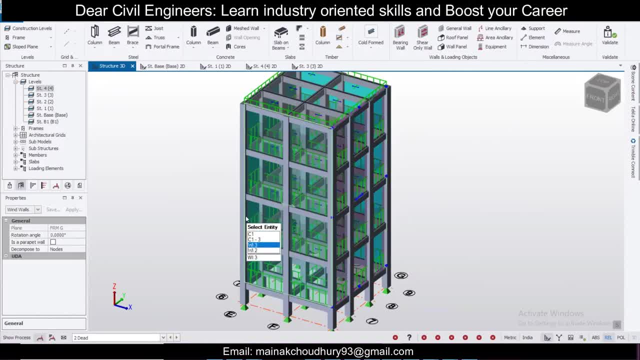 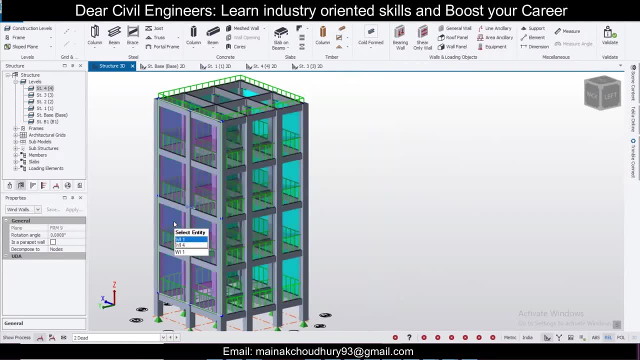 so we have, you know, selected this particular wind panels and can simply select decomposition. you know, nodes, members and rigid diagrams. there are three options here. so do this as rigid diaphragm and ignore diaphragm here. also, make this as to the diaphragm and no diaphragm here, because you don't want to consider. 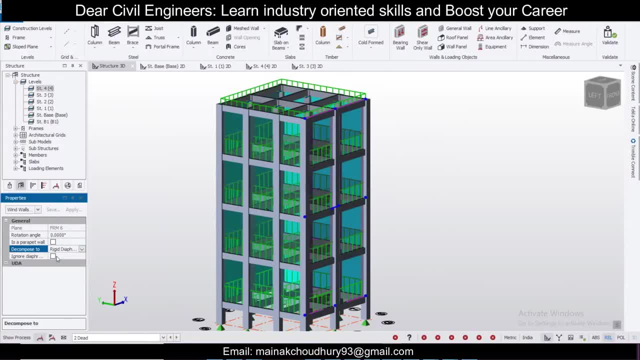 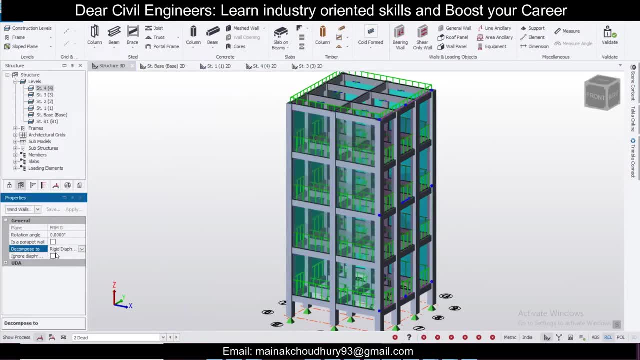 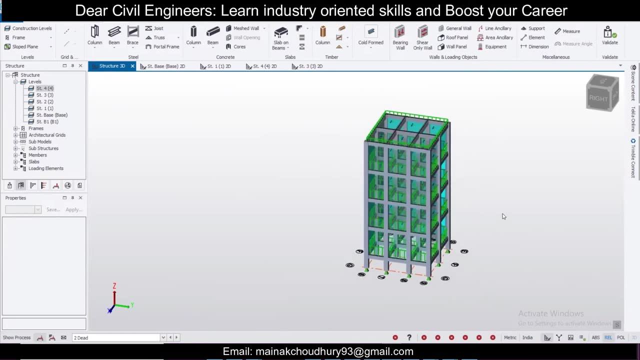 this as the loads here you don't want to consider, just for you know, taking the wind loads, we are considering this as diaphragm. so if they have come, and you know that, so we have done, you know, on all the four sides the same thing- uh, what you do? just validate the model. 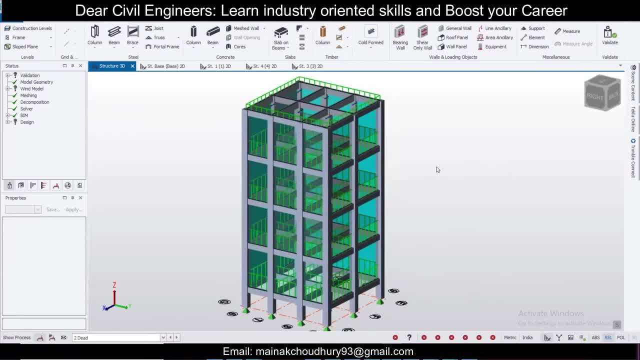 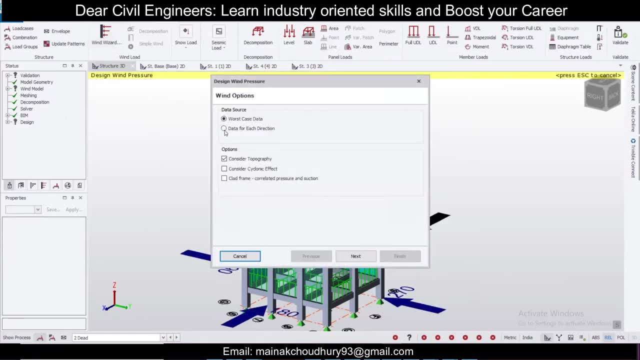 check whether everything is okay till now. so when everything is okay, just go to load here and open the windows. so worst case data to be considered and uh can ignore this. consider topography or consider cyclonic effect. if it's in the cyclonic zone, you can consider this, or if it's not. 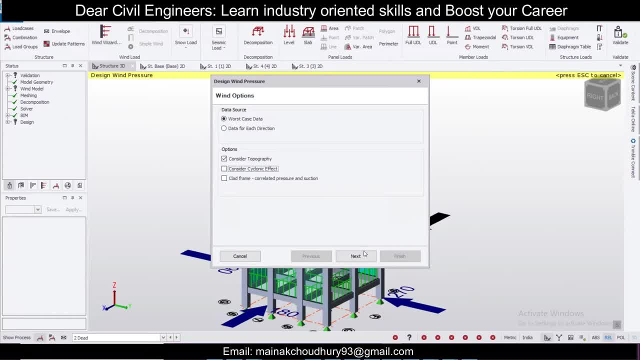 in cyclonic zone. you can uncheck this and uh, just click on next and orientation. here here give 90 uh, which means that the wind will act. you know, 90, 180, 270.. so around the 90 degrees it will act. building height exposed to wind: maximum height your automatically takes and then the basic. 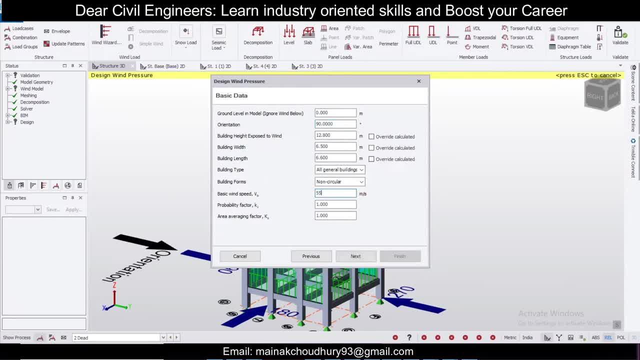 wind speed is your 55 for tripura and uh. i have already shown in the. you know we don't win uh. the of the is code 875, part 3. you will find a table and also a map in which basically speed is uh located and k1 and k2 factor will be one here for tripura and again the detailed part: why this? 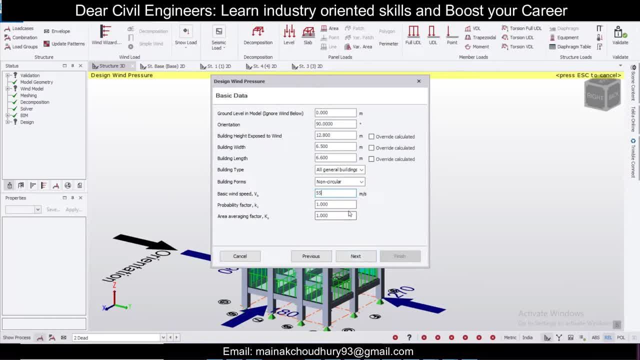 one you can find out in the video on the tips part. so this is the same thing. so I'm going to repeat this. not going to repeat this, but basically you can just go through is875, part 3, for those factors. just click on next and the terrain category. 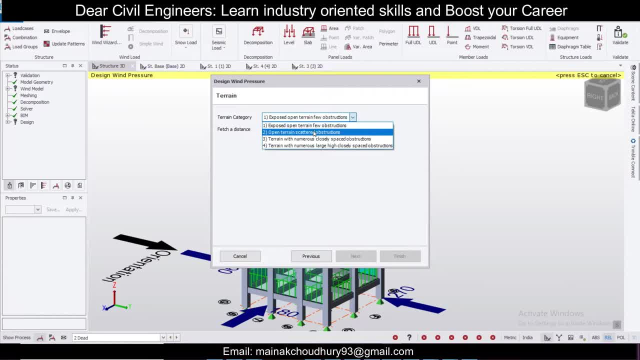 uh, you know exposed terrain with few obstructions and terrain with numerally numerously closed obstructions, so we're going to go with open terrain with scattered obstructions. fetch distance is basically the distance where the wind patterns are the same, so I'm going to go with five meters. 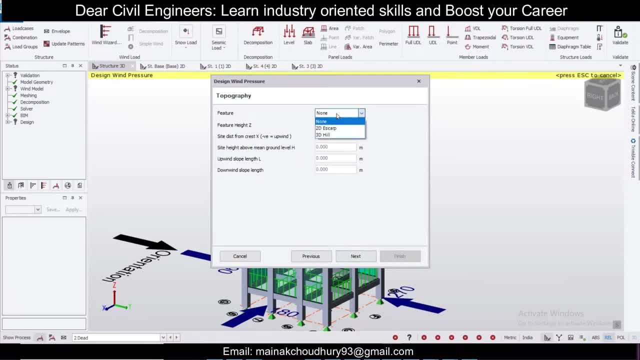 so this topography feature, you can take any topographic feature, or or you can also ignore this. if you will ignore, this is considered none. um, generally, you can ignore this. so just click on none here and then next. next, so you can see the k1, k2, k3 and k4 factor. they have taken automatically from. to change this, you can- uh, you know, change. 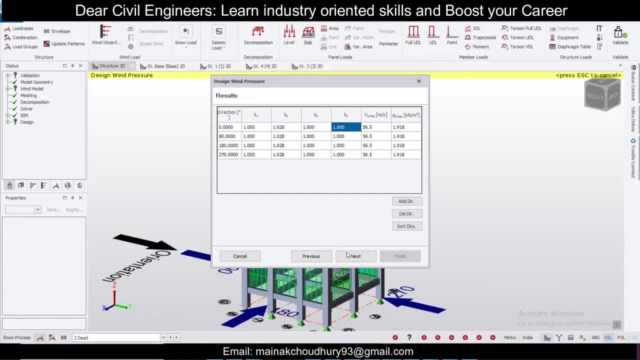 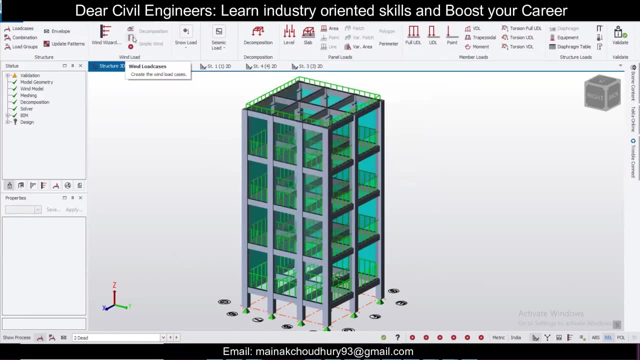 this also. there is an option, but now we don't need to because already you have considered all the. so the design, wind speed they have calculated, then click on next here and then click on finish, so after that you can see this, that the cases and update zones, and then you have this: delete wind, so win, load cases. we click here and 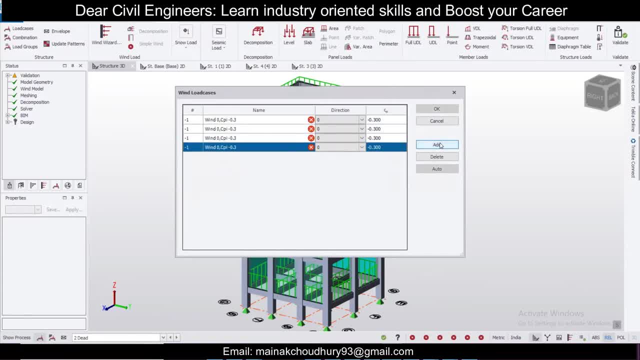 can just click on add here. so four win load cases they have taken here and first go with zero, next with 90, and then with the 180 and then with 270. so the cp values they have taken you know automatically. you know 0.3 they have taken. here can edit the name, but, uh, the cp values. 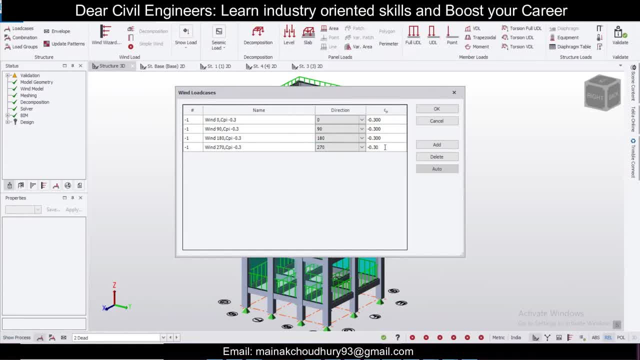 which they have taken here. they have taken automatically. if you want to edit this, suppose: uh, this is the wind zero which is coming from the zero direction. so this is basically uh. as we know, this is basically. you can take this as 0.8 and from the lever side, that is the 90, you can take this as 0.5 and similarly for the 180, you. 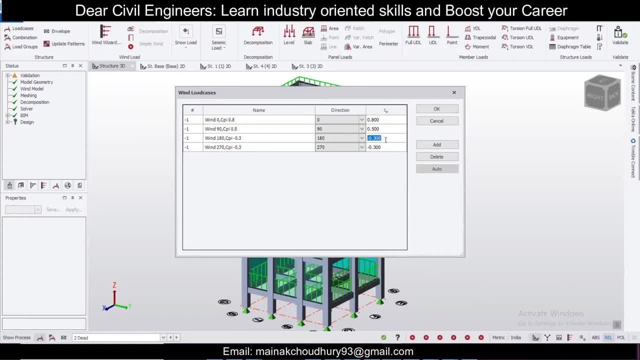 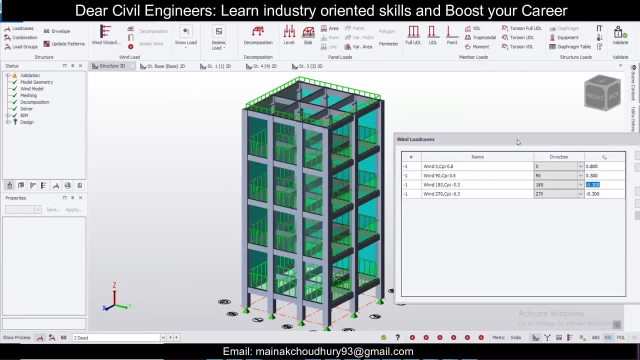 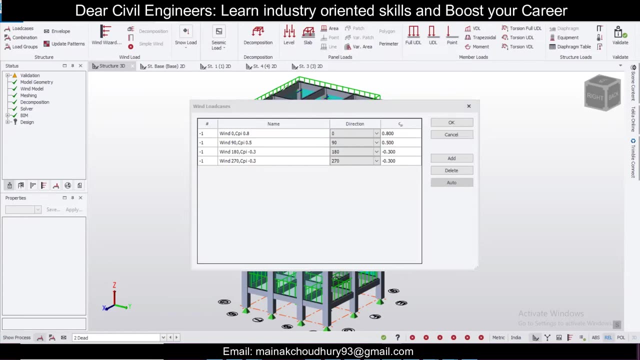 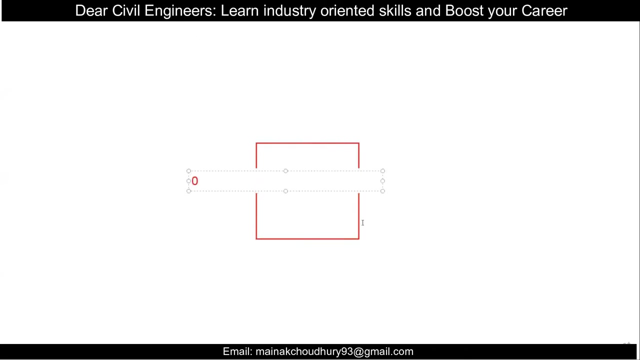 can take this as your, this 180. you can just check here which direction will be the 180 here. so if you just check here, in this particular, you know, let me draw a rectangle to explain. so if this is the 0 and this is the 90, and if in terms of axis here, 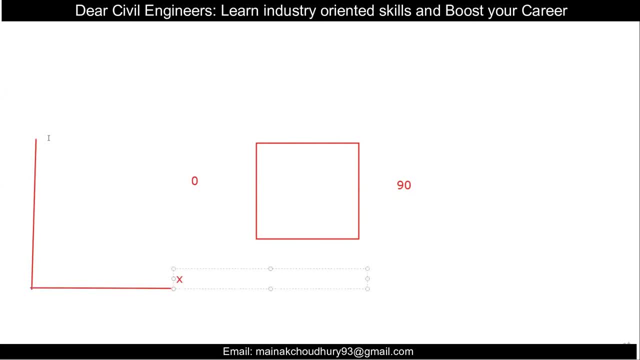 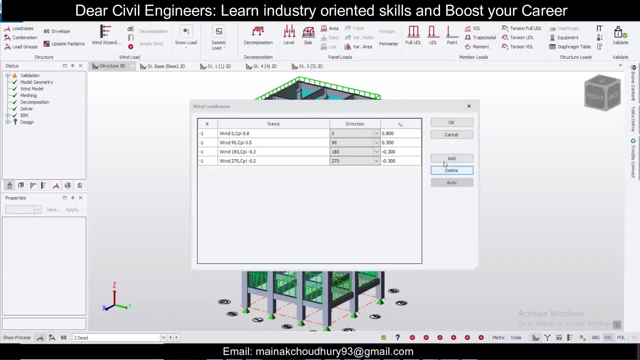 and this is the- you know, x-axis and this is the y-axis. so, uh, here, if you want to see, here, this will be 0 and this will be 90 and this will be your 180 and this will be your 270.. so, coming, it will be like this: you can just verify, you know this, uh, properly, you can just go. 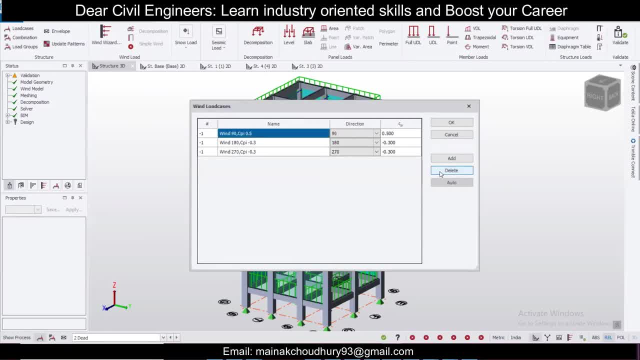 here and uh. first of all, i'll delete this, all these combinations, and click on auto. so so we are going to add some wind load cases. just click on this window case and this wind load case is now here the possibilities. here are only examples of wind load cases. 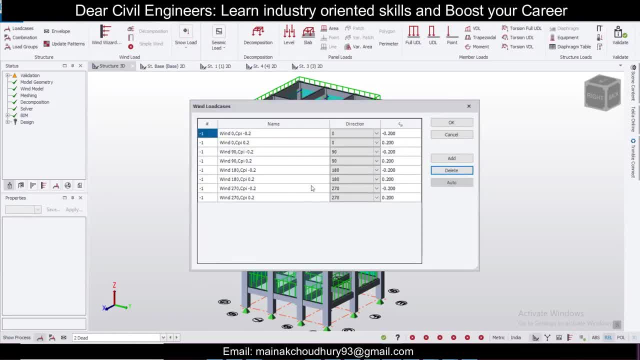 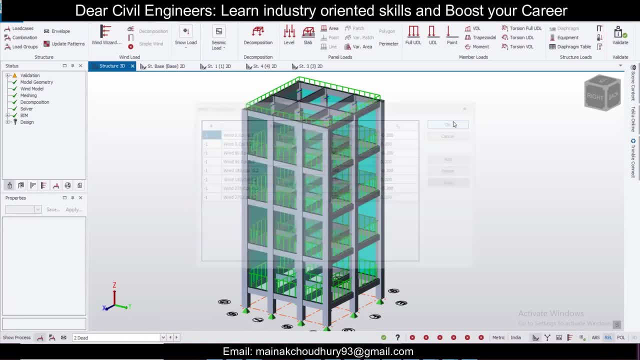 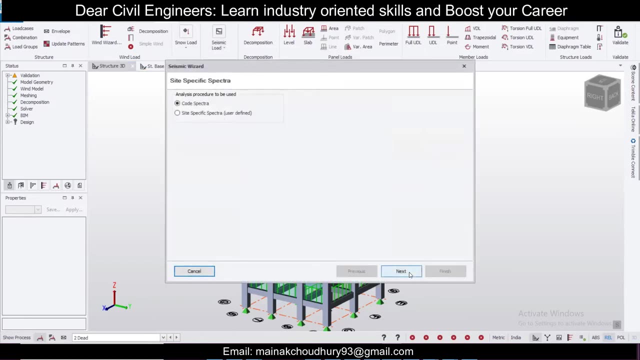 win load cases. you can add this manually or just click on auto so the cpi values you can see automatically in it, as we have inserted manually. so then you can just click on ok. so after that for the go to seismic load, go to seismic wizard and then code spectra and just make this ignore. 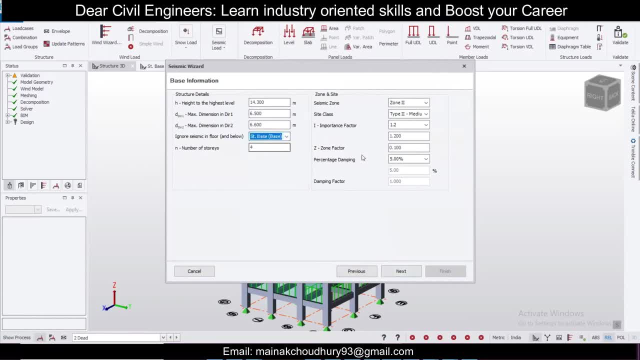 seismic below our print level. this for this case it's texture base and then zone i'm going to design for tripura, so it's in zone 5 and this is based on the is 1893 2016, part 1. side class is medium importance factor is one for the residential buildings. again, if you check utah's. 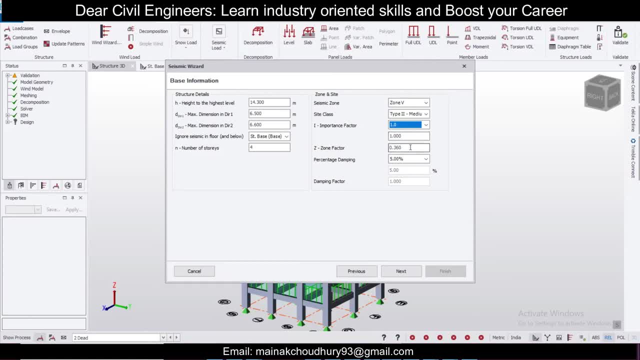 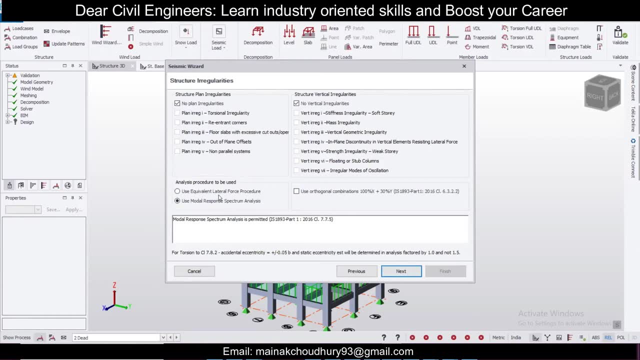 videos on the seismic. you can find out the detailed is code explanations if you want that, and then damping is okay and you can have two options here. you have this equivalent lateral force procedure of the model response spectrum analysis. i'm going to use this model response spectrum analysis and then click. 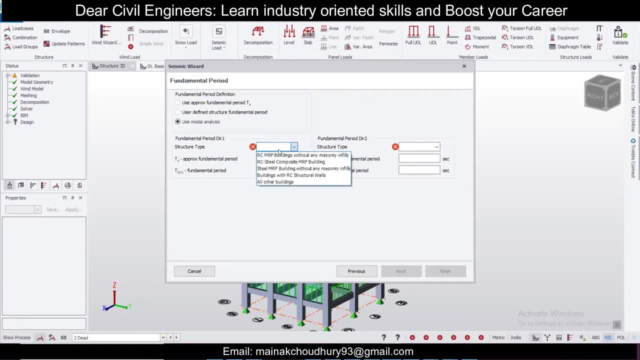 on next here, structure type, you can find out here you have this rc moment resisting frames, rc steel composition frames, buildings with the rc structural walls and all the buildings. so we're going to select here rc moment resisting frames here, and then click on next, and here also you have this moment frame systems. 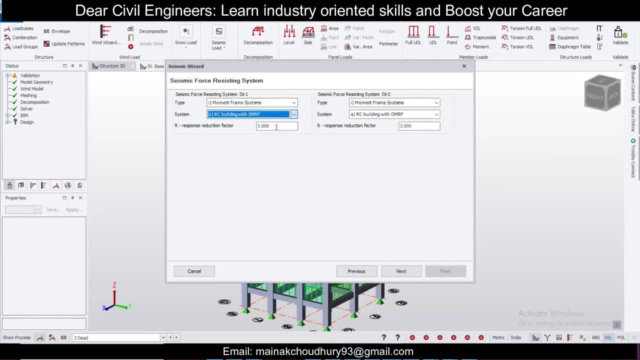 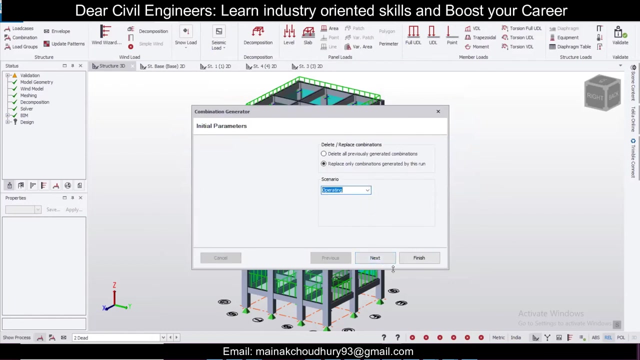 here also momentary systems. you can do, say select here i'm going to select rc building special momental sting frame here- and then click on next. select all these import load and dead load- i know the system takes into consideration- then click on next, then click on finish. create some load combinations according to the seismic load. click on next. 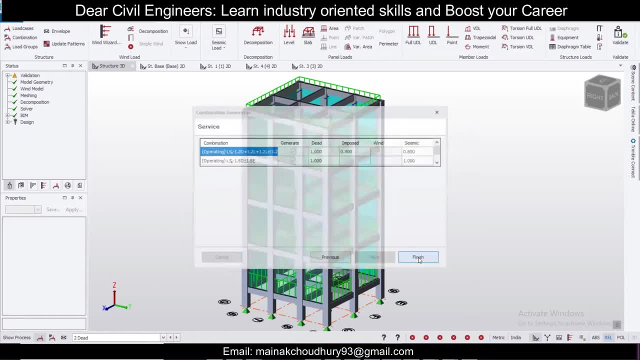 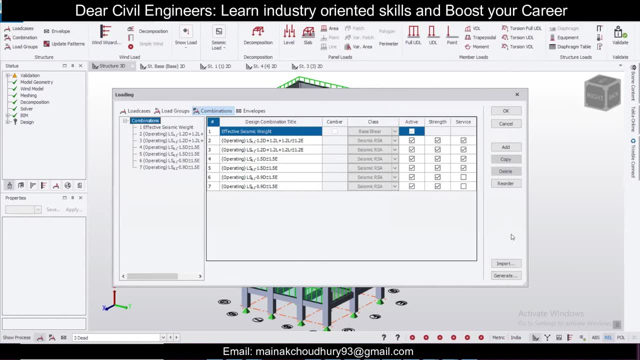 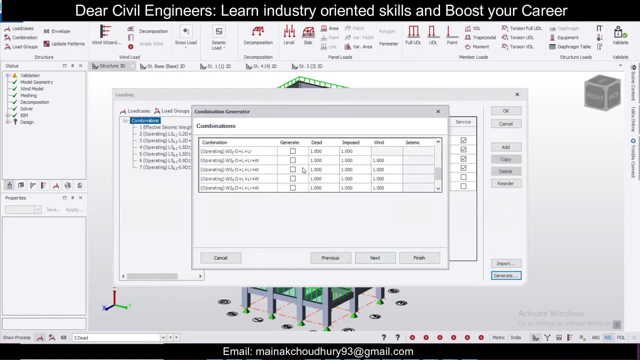 the widget combinations have been selected automatically. next and then finish. lastly, we'll go for the load combination as per the is 875, part 5: clicked on combinations and click on generate, next select this and these are all unselected. these are working state uh stress method: load combinations. click on next, next finish and okay. 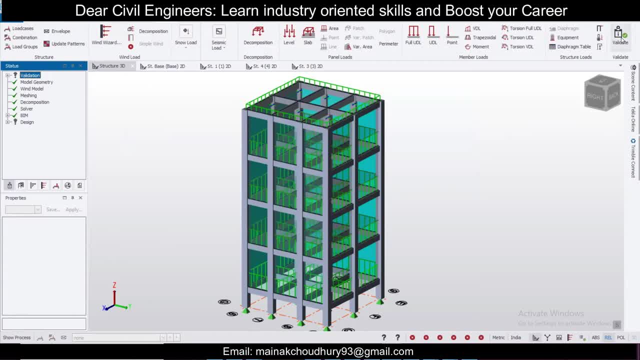 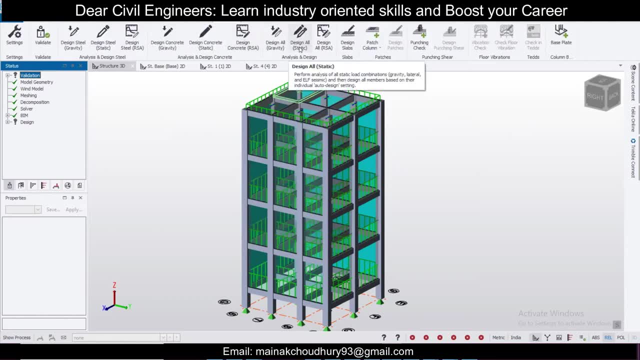 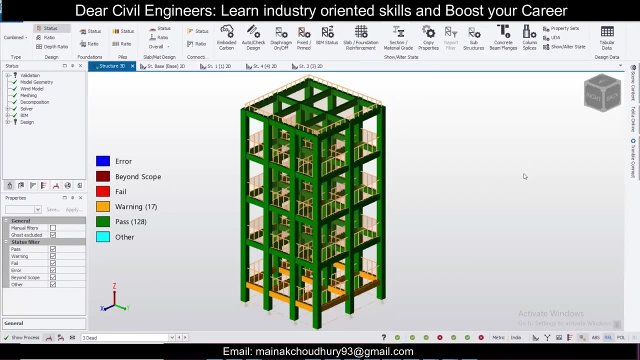 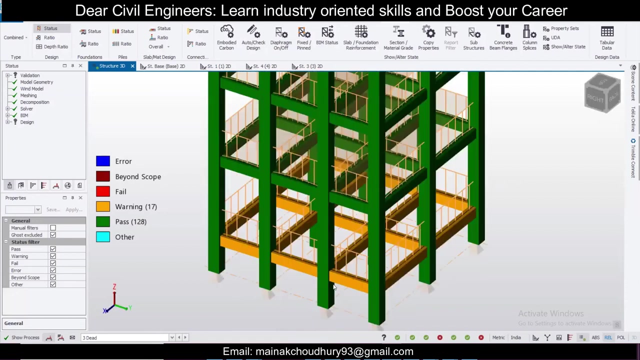 click on validate to check whether everything is okay in your building. so once you have done that, go to design and click on design- all static, so, as you can, the design has been done and all the members are safe here in to design my is code. there is a you know, a little bit problem. that warning comes, but you can ignore this. 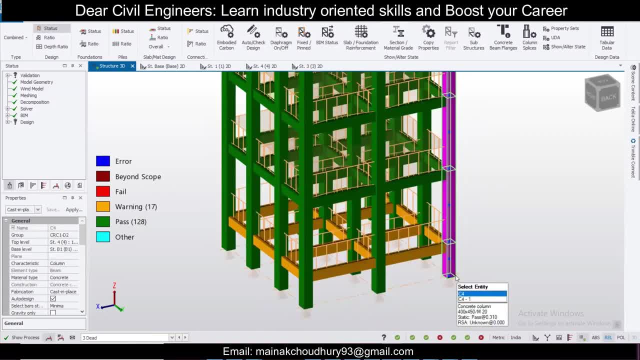 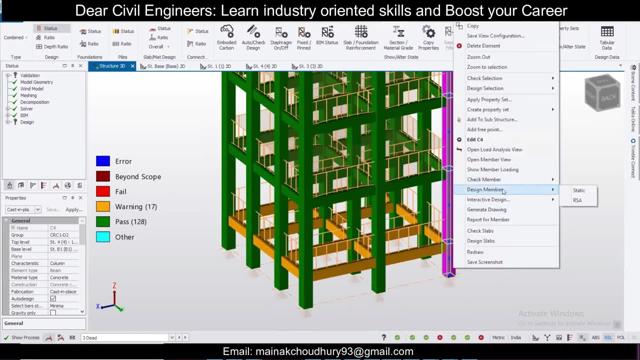 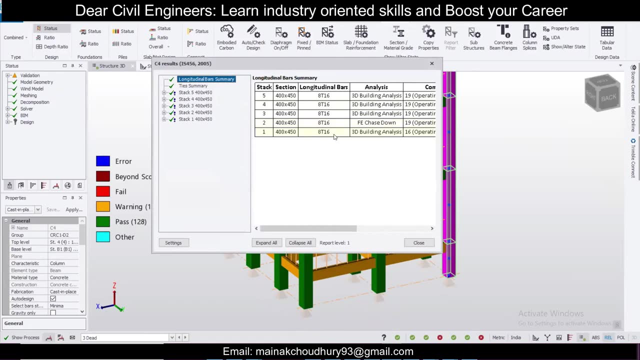 for the print level. basically all the members are safe here to see where any design here. suppose for this particular column. what is the design here you want to see here? so just right click on this particular column and you can just use the check paper static and you'll see the results. here you can see eight bars of 16 mm has been used. 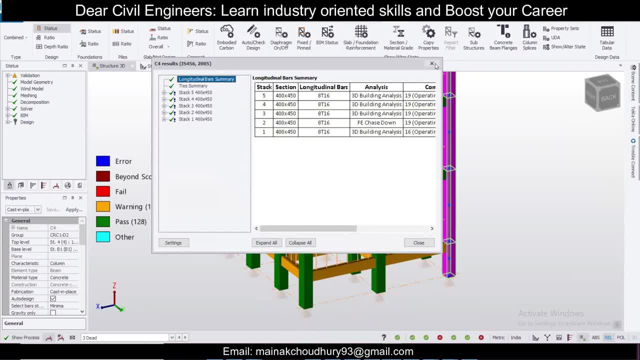 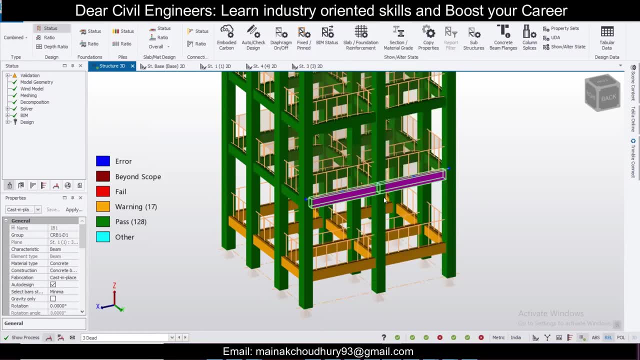 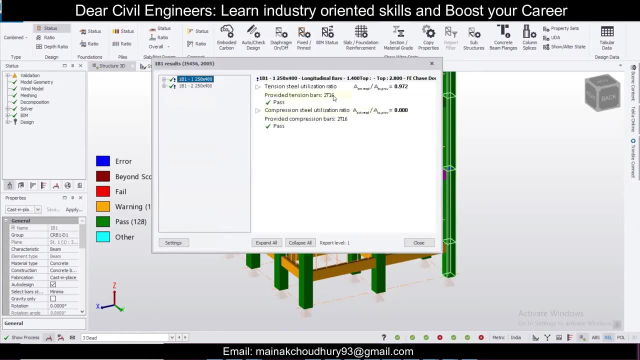 right from the you know bottom to the top story and uh, everything's safe here, suppose for this particular beam. you want to check the result here, just select this particular beam and right click and then uh can go with. uh, let's see check number static, and you can see here two bars of 16 on the top, two bars of 16 on the bottom for 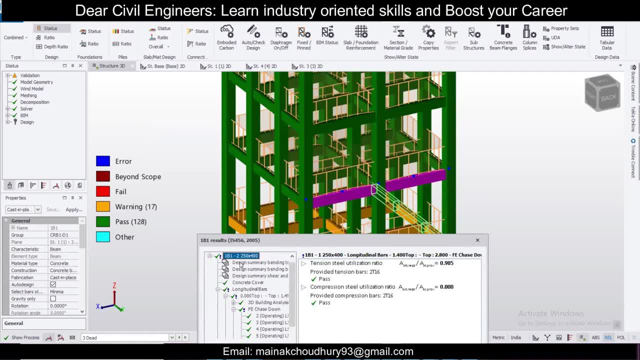 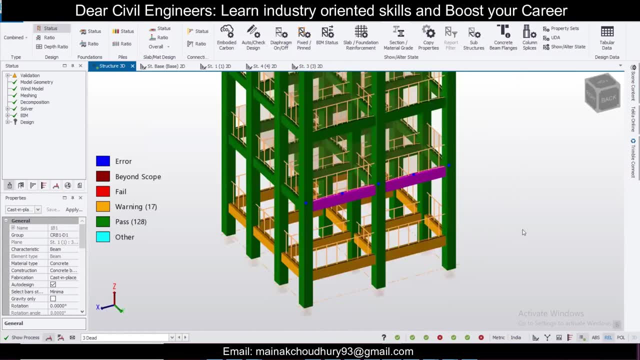 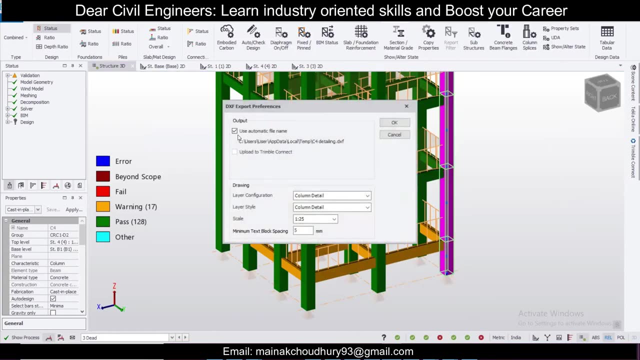 the first span, also the second span, and for the first plan, or this is the second span, they have used the same thing. so like this you can do, and if you want to find out the drawing of this particular column, you can just right click on this and you can see, click on generate drawing. 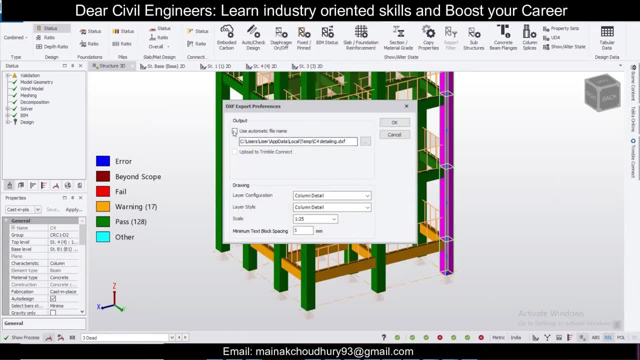 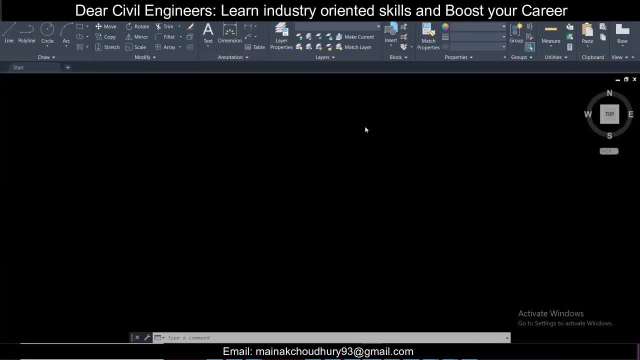 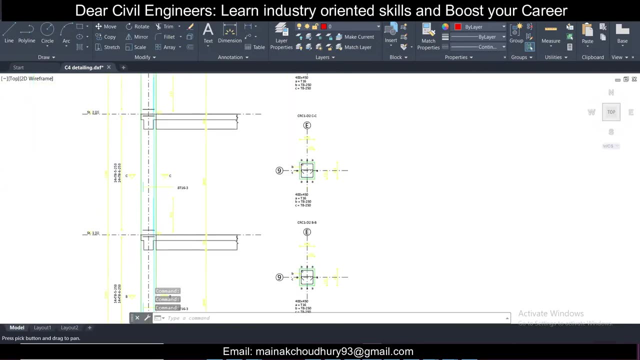 and if you want to give the location, just keep the location here or to the default location. so click on ok and you'll find the drawing which will open directly in your autocad. so this is the drawing which is opened directly in your autocad. you can see the drawings here, eight bars of 16. 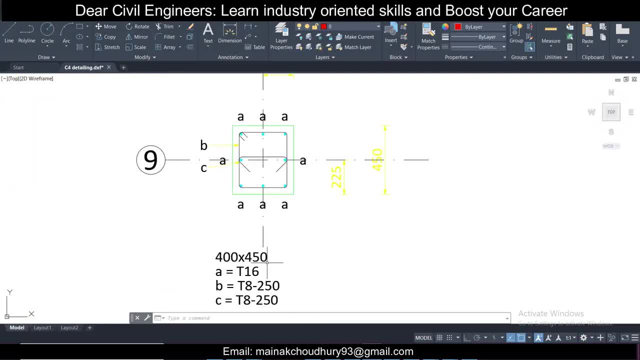 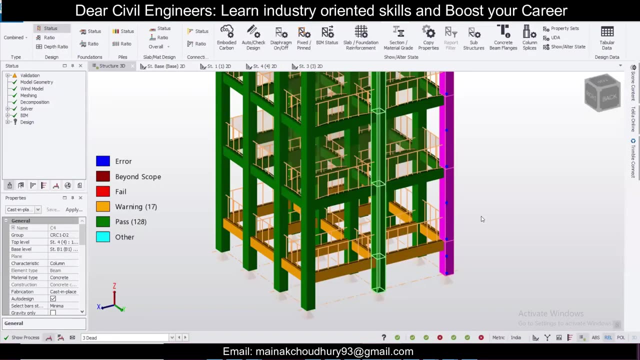 mm. and if you want to see the tie detail, the tie is also spaced, placed here at 250, center to center the tie distance a little bit more, but you can see the drawings have been generated, along with the bar quantities also, so it's very helpful. and if you want to design the foundation here, just 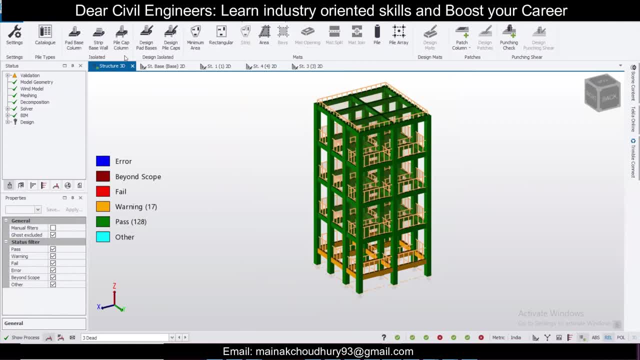 you can go to your option of your foundations, go to pad base columns and if you just insert the sbc here, you can find out the option of your complete class and then your other things as well, and here you'll find the soil parameters. just insert the soil parameters according to your soil test report. 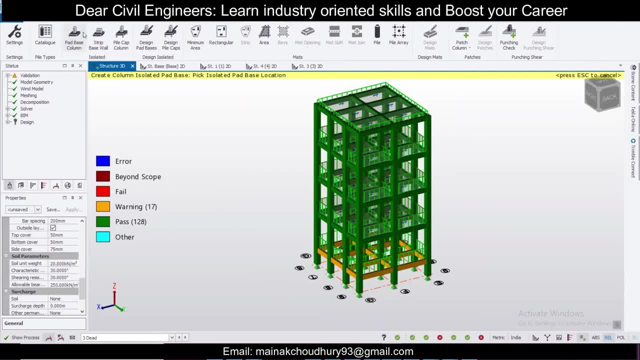 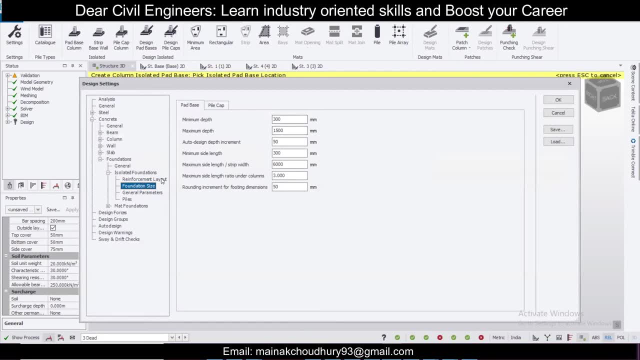 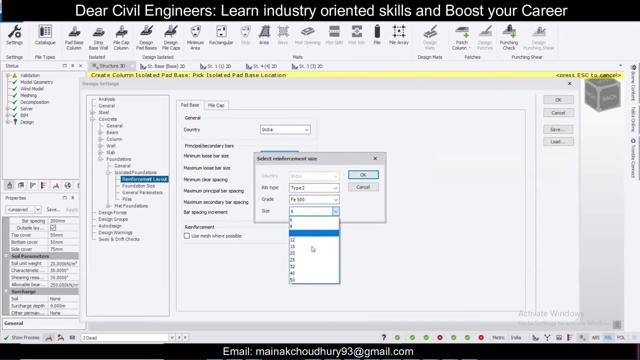 lbc and you know soil unit weight you want to change and you know, go to the settings and in the settings if you want to change anything, you can do that, like the reinforcement layout, the minimum reinforcement, maximum reinforcement, uh, you can just change that. changes to 500, uh, 10 mm. 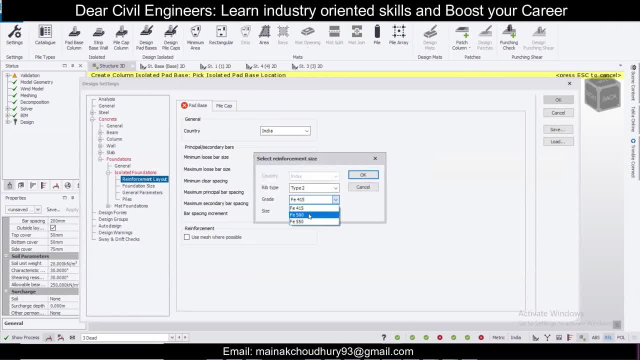 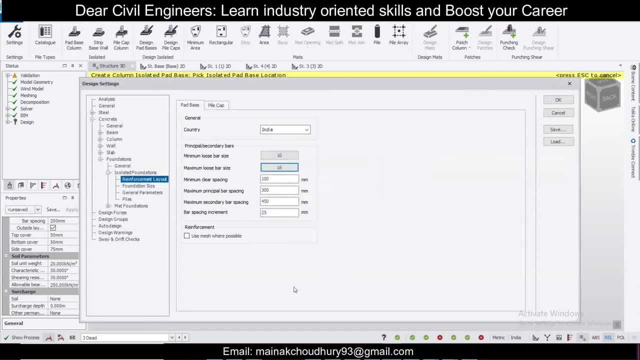 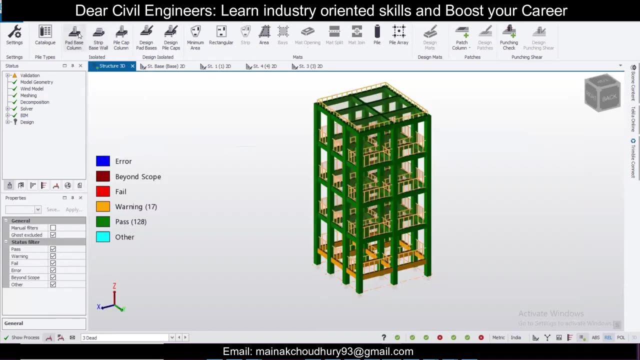 let's go, and the maximum also at 500, and you can do that. you can also change the setting of the soil parameter and then you can go here. let's go here, 16, click on ok and then just click on ok, here, okay, and then go to pad base column and once you have inserted 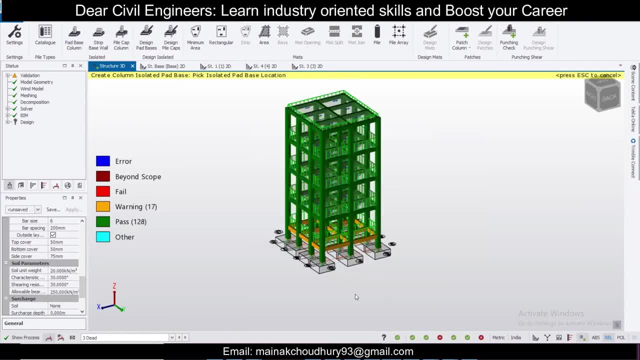 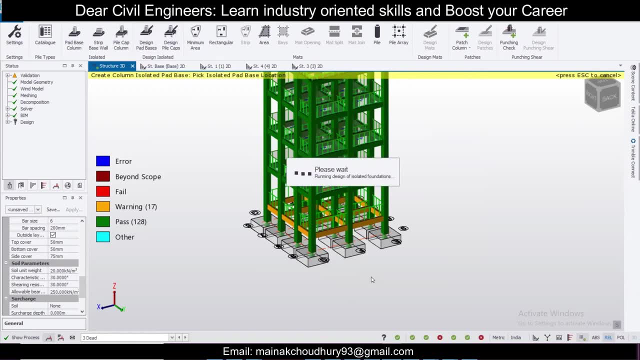 this and also soil parameters. just select all this entire thing and then click on your design path. basis pad bases will be designed. so a warning will come here if you are designing with is code, but if you are designing with any other code, the warning will not come. so this is basically glitch. the warning of development link. 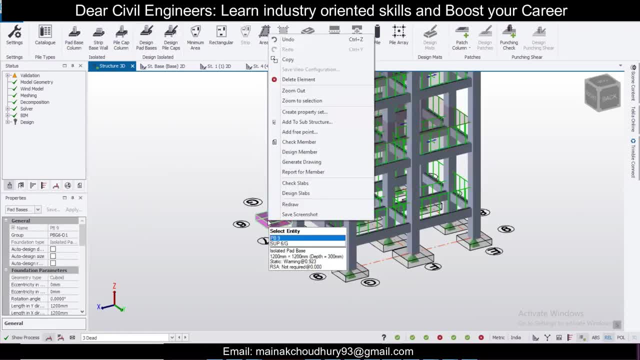 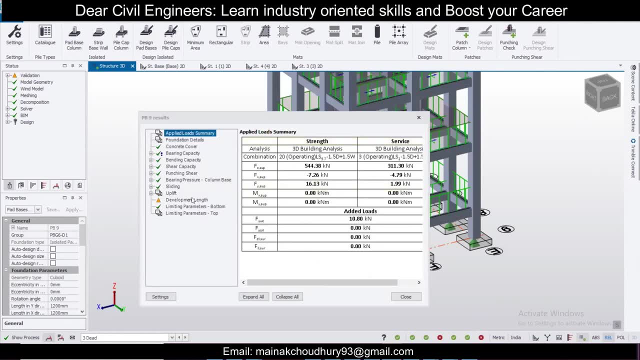 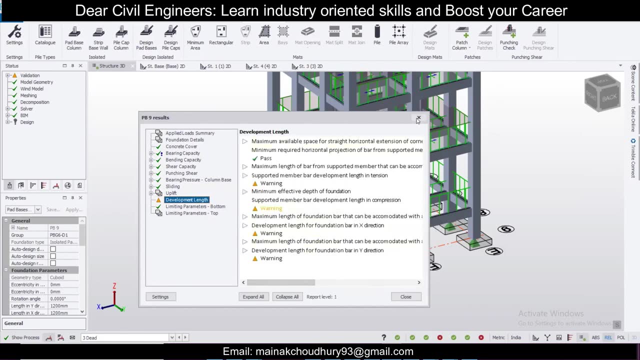 comes. we can show you here. you can see here, check, check member so you can see development length. warning comes. this is uh due to a software, at least so you don't need to worry about that development link already they have considered. but uh, the beauty is that the foundation layout you can find out and economical. 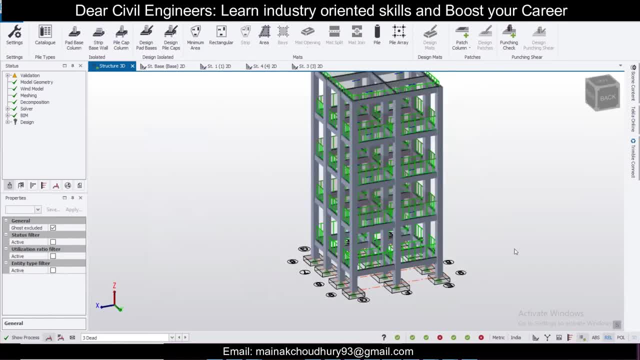 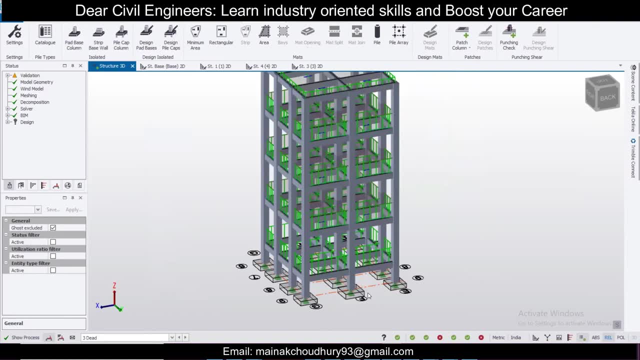 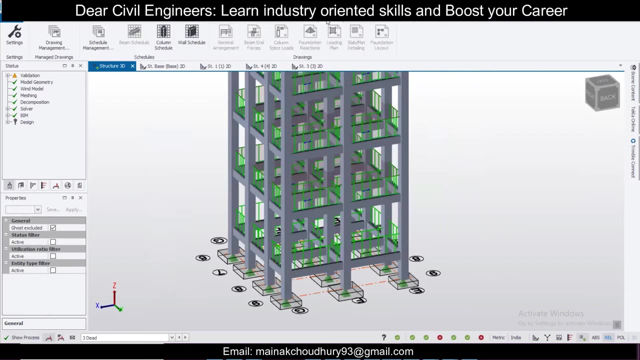 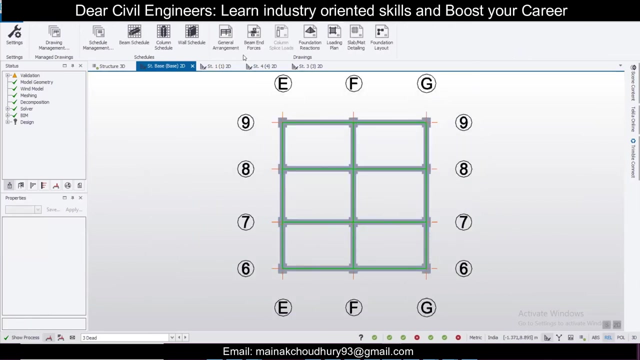 bad footing. designs also, you can generate. so let's go now to the generation of report and generation of drawings. you can take a break and then you can come back. so welcome, after the break, go to draw and go to this our, you know, base or the length level, and after that first drawing which you are 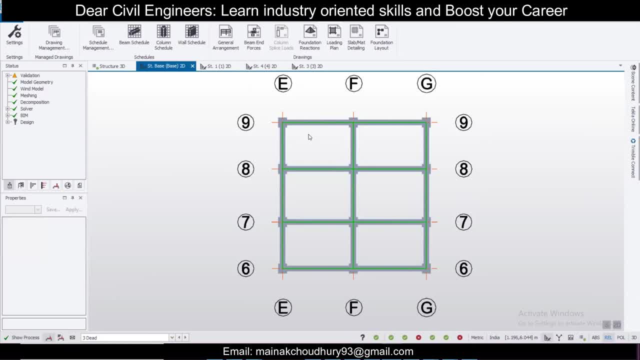 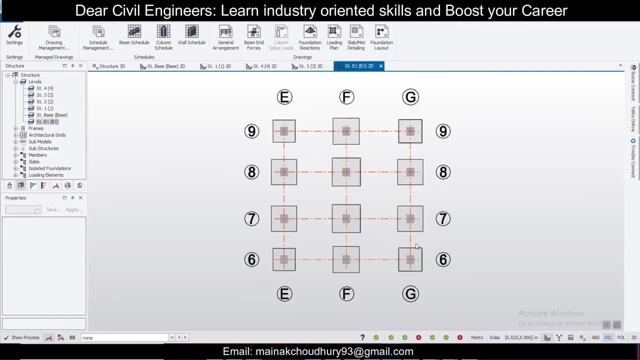 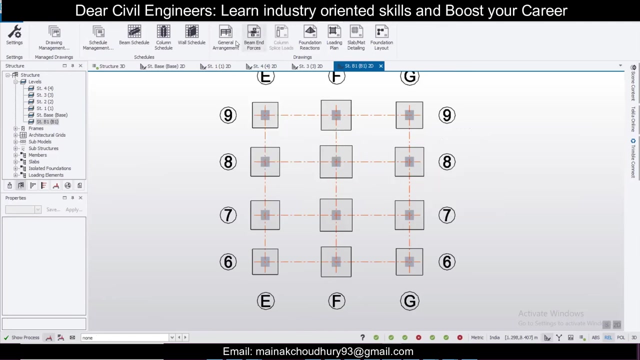 going to find out is our column layout. okay, so, uh, we're going to go, let's select this structure to the bottom, most level, and here only the foundation and column are present. so so we'll go first for the column. you know, layout general arrangement will select and, uh, this time, 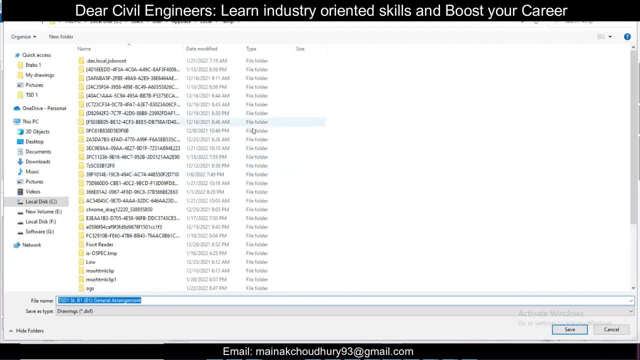 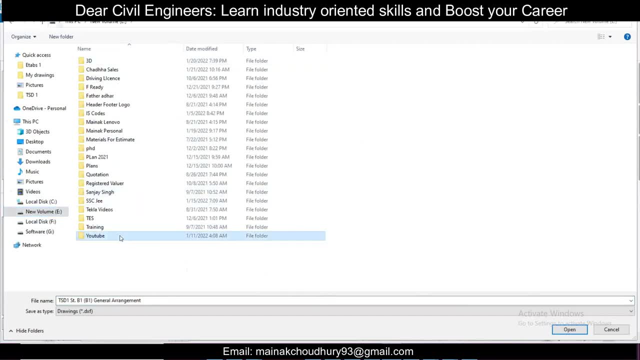 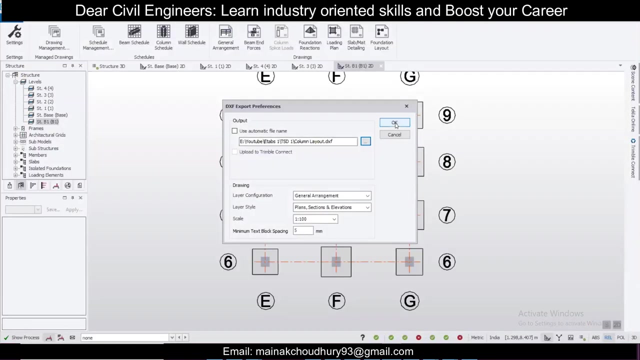 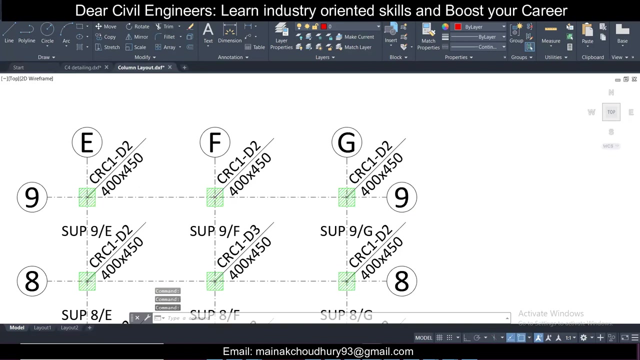 we'll just select a particular place for you know, storing everything. i'll select a particular my location here of the video and let's go here. this will be our column layout. okay, now layout. so click on save, click on. okay, so this is my column layout. i have all the names of the columns here. 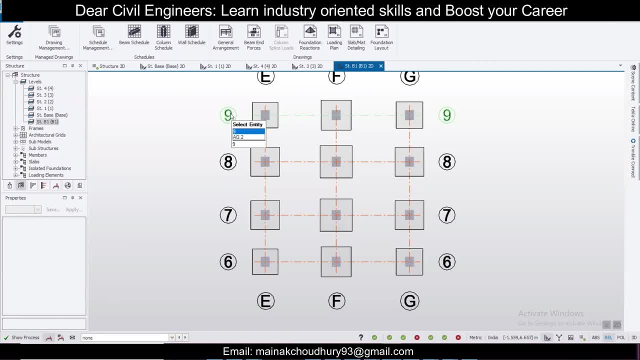 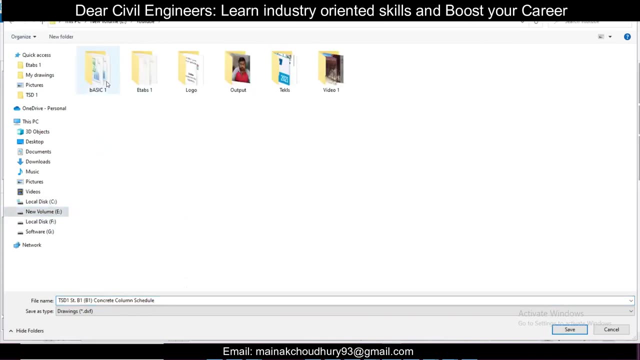 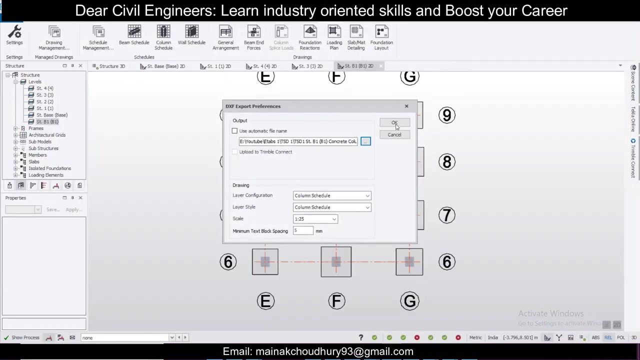 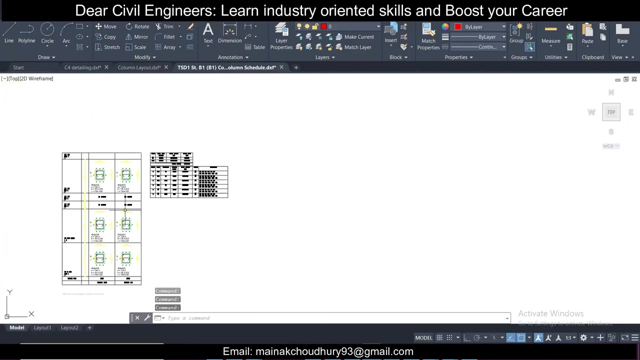 and next thing which you need is the column schedule or the column details. so just click on column schedule, click on. just change the location here to whatever location we want. concrete column schedule name is okay, just click on. so we have the column details here, the reinforcement and the details which has been used, as you can see here. so column details, we have found out. 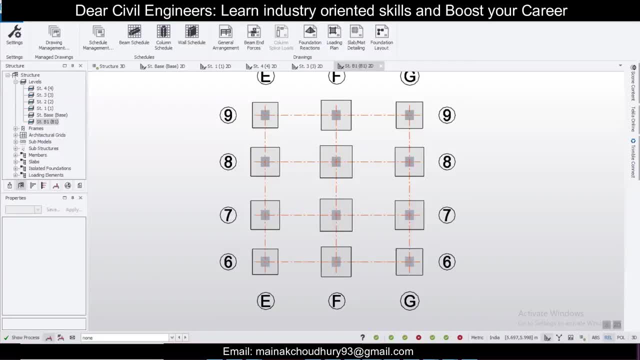 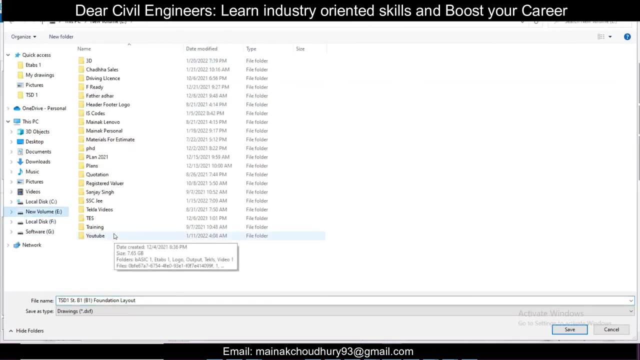 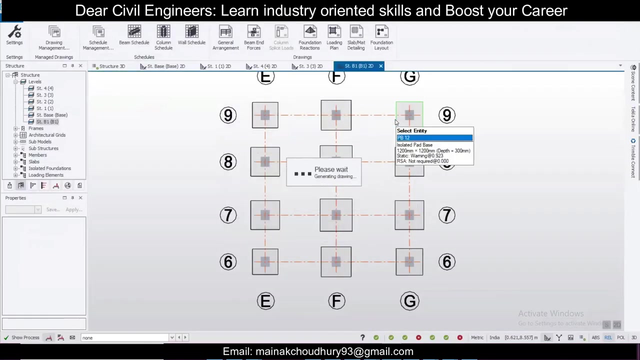 and the column layout which we have found out. next let's see, uh, find out the foundation details. so we go with the foundation layout, change the file location here and to our location, foundation layout. click on save. okay, so we have this foundation layout. as you can see, unlike stat flow, which is a very you know- 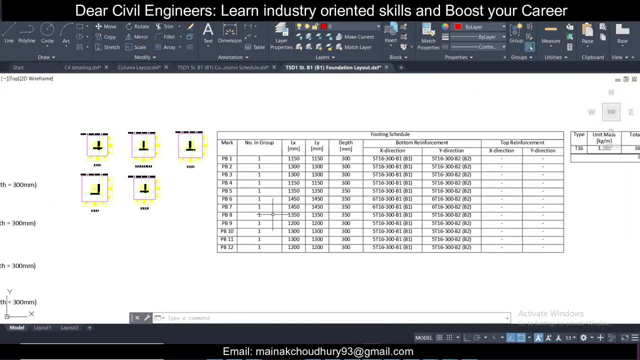 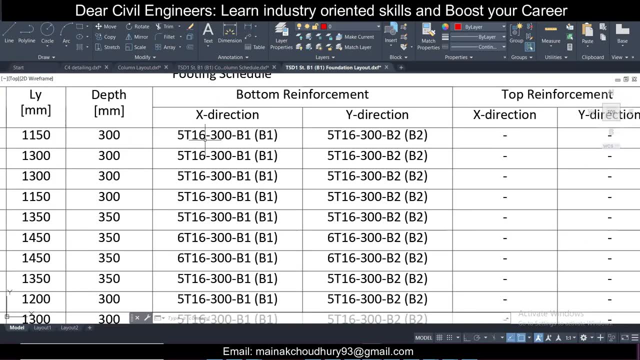 economical design, as you can see, for the foundation. see, this is a very, you know, economical designs for the foundation. they take the unfected loads so, as you can see, five, sixteen on your bars, three hundred percent. so this is very economical design for the foundation, that's. 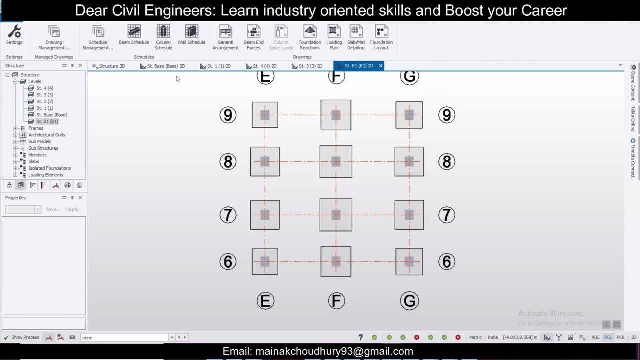 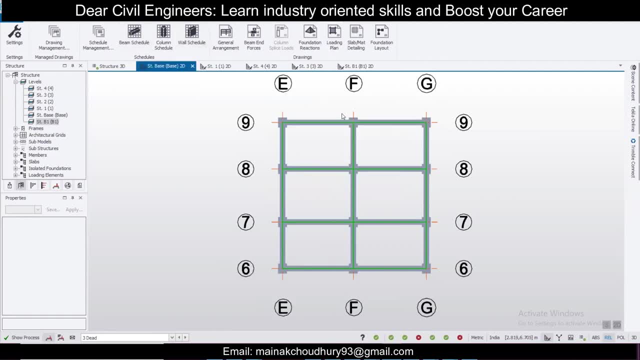 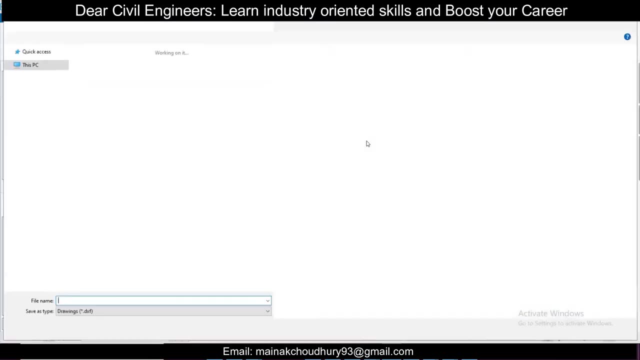 what is the special feature of this software? now for the next beam column plan, let's go to structure base and, uh, just uh, you can find out here the general arrangement drawing, and then obviously, just give the file name, and this file name will be your length, we give your length. 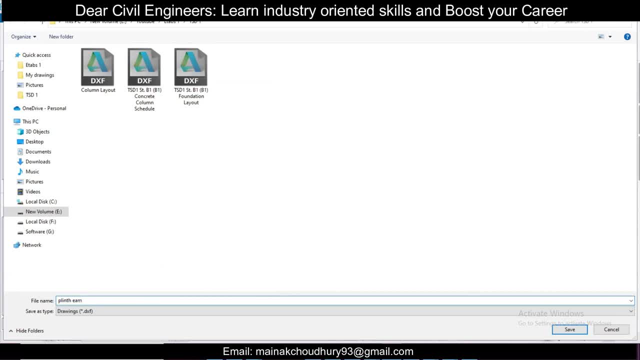 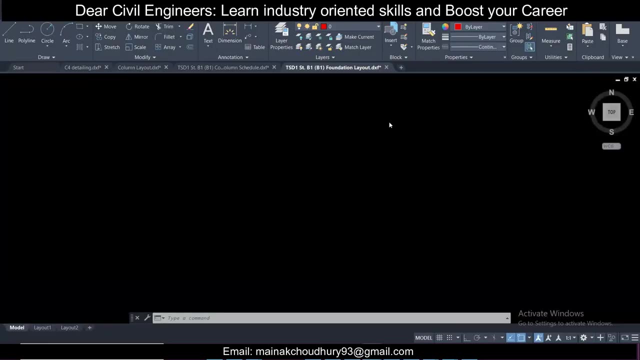 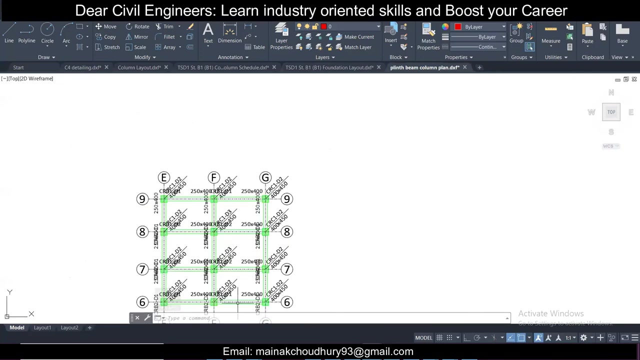 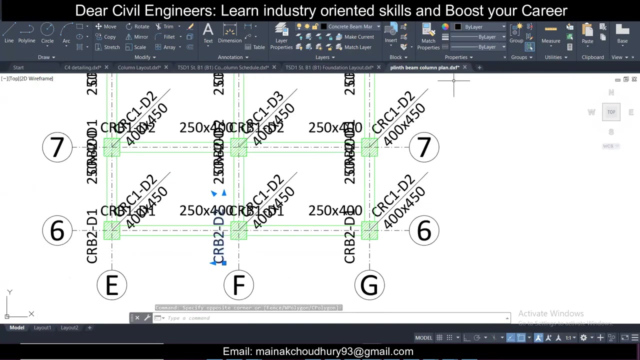 beam column. let's click on save, click on okay, so we'll find this uh clean beam column plan. if you want to do the beam details, you can also find out some of the projects of you know the beam details of cr b2d2. so for that you have to find out the beam schedule. we just go here and 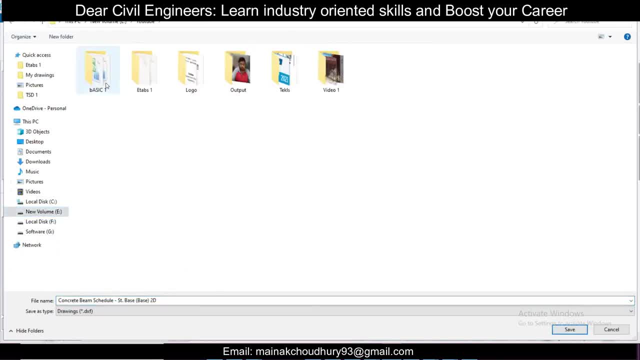 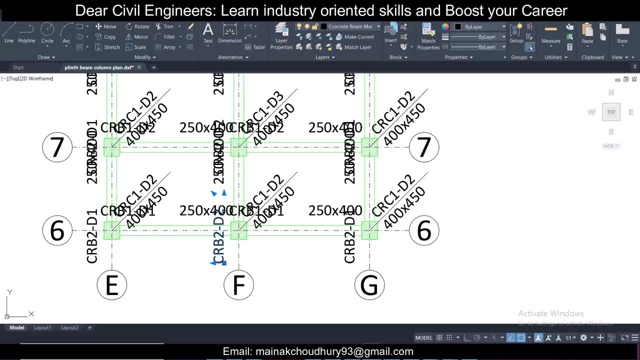 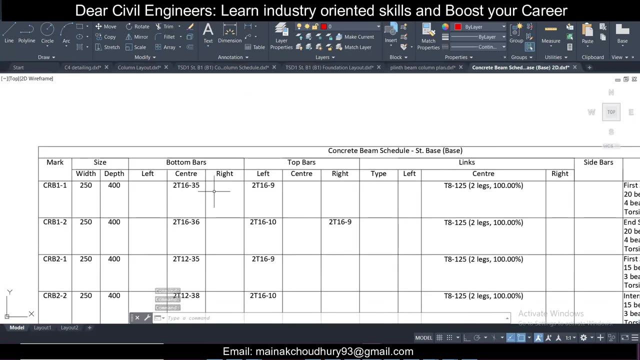 just insert the beam schedule and just try giving the location see click on okay, you'll find the beam details. this is the software calculates. as you can see, these are. this is the beam details: bottom bar 16: uh, two bars on 16 mm and top, also two bars of 16 mm. 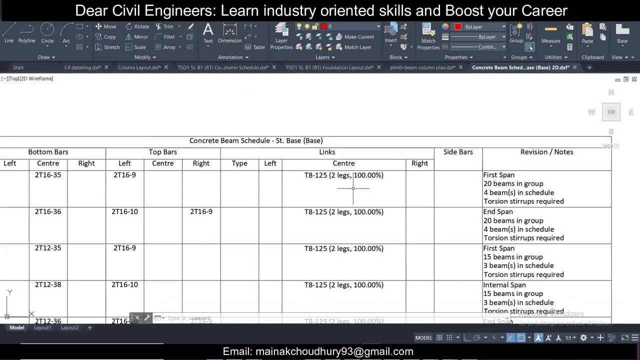 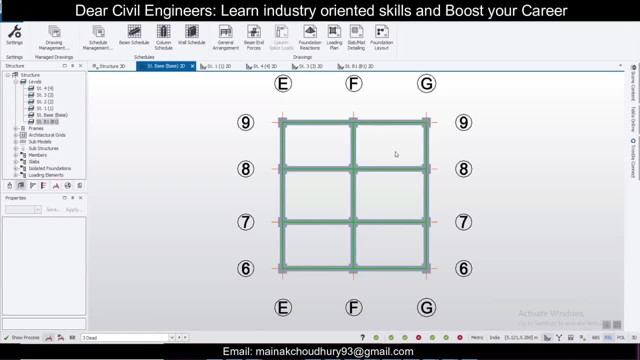 in the stirrups: 8m stirrups at a spacing of 125- so pretty you know. economical, practical design the software has given. so like this we can find out for the remaining floats as well. so now i'll go to the report here. if you want to generate the report and, uh, suppose, all this report. 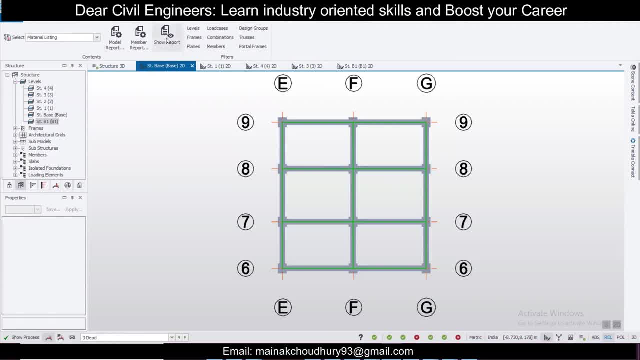 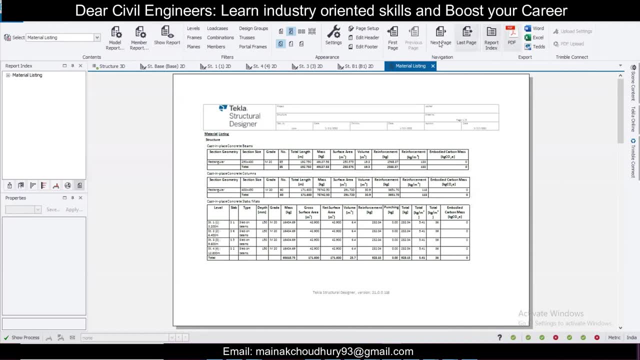 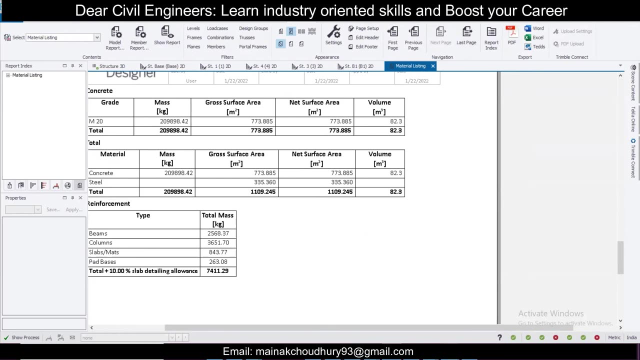 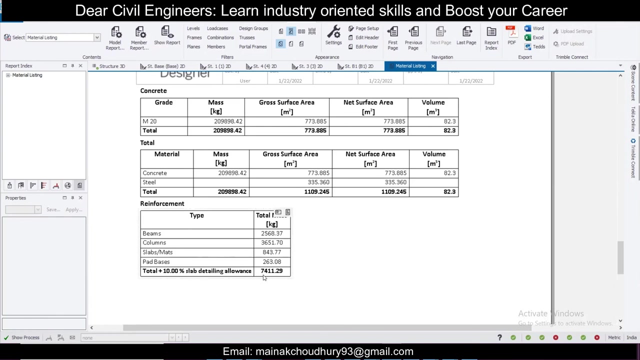 you can generate. suppose i want to see the material: take off material like material listing, and then select show report, convert it into pdf. i'll go to the last page and i'll show you the total quantity which has been used here: reinforcement: 7.4 tons unit in this building. uh, the rebars and the concrete, you can see 82.3. 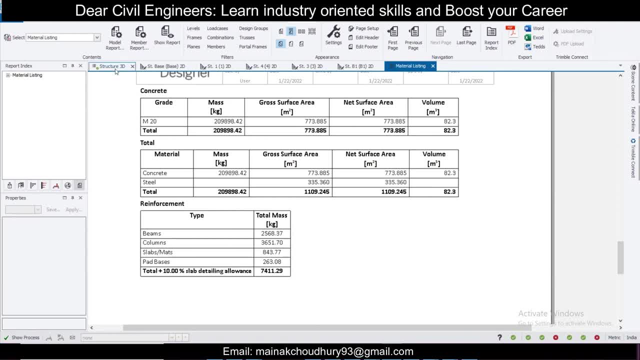 meter cube. so, again, this is very helpful, uh, and also you have the other reports, you can find out the building design and you can see the building loadings which you can submit. if you're, you know, approving this building from a government, you can use this and, uh, just click on this pdf option and then it will be converted into a pdf. so 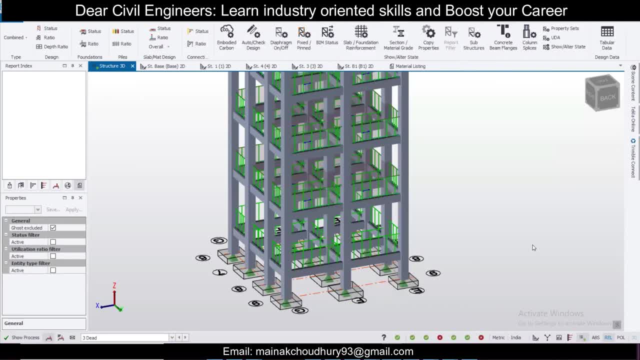 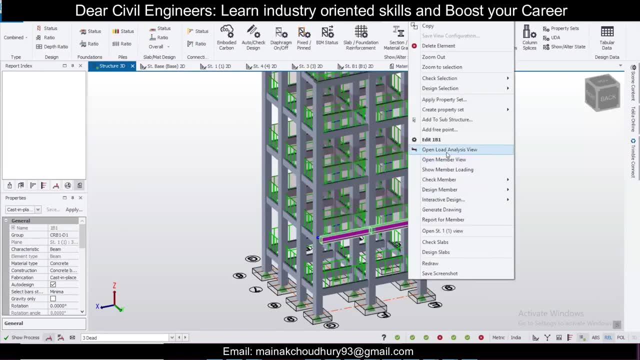 these are the things which you can basically do and if you want to see the- you know- bending movement, shear force for any particular beam, just select a beam and just click on open load analyzer view. you'll find the bending moment and shear force diagram of that particular. 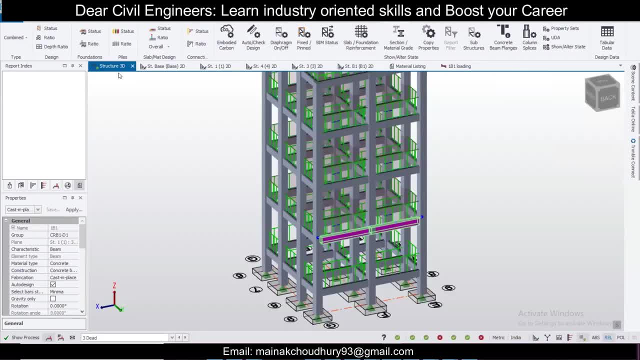 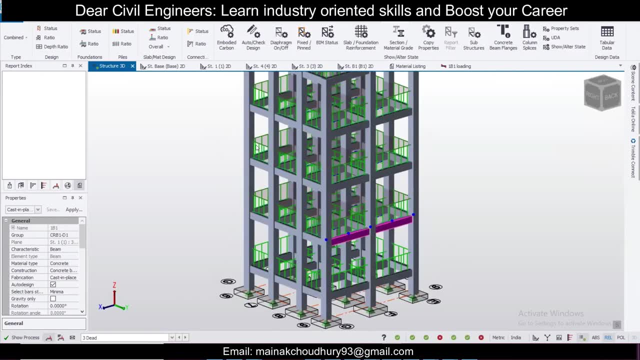 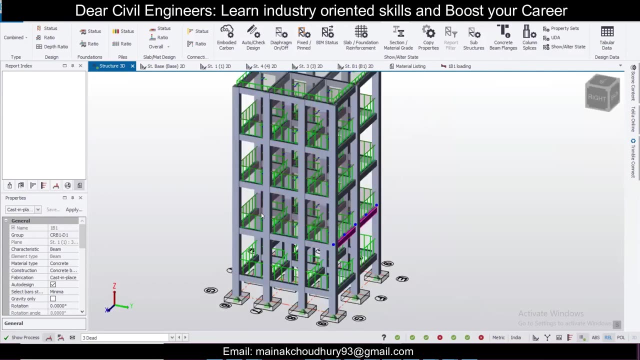 uh, you know, beam, uh, going back to your structure 3d, and uh, there are a lot of things, other things which you, which you can do and which you can check, and uh, this, those things in detail, will make videos on that and if you like this video, make sure to leave a like. and 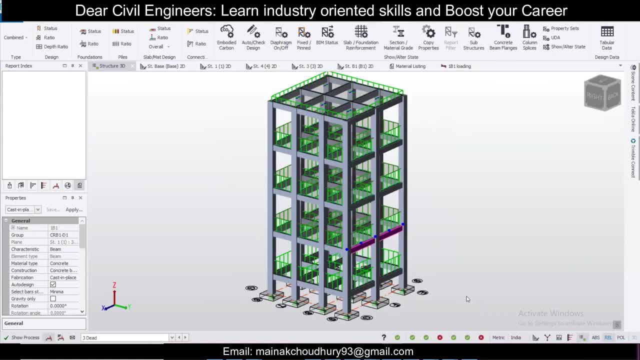 keep learning wherever you are, stay safe and stay happy. bye.